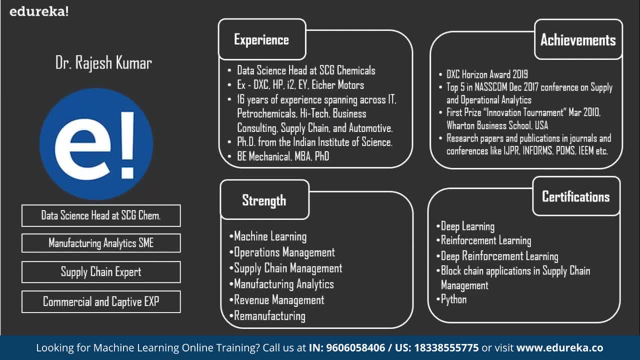 So I was part of the captive analytics setup at HP where I used to lead a team. in terms of my educational background, I am an engineer, a mechanical engineer, from NIT Bhopal and I've also done my MBA and PhD from Indian Institute of science in the supply chain and operations management area. 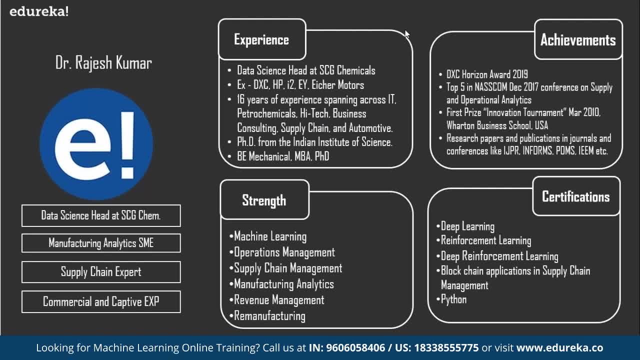 you know, I worked on a project and my team. we won the first prize at Innovation tournament held at Wharton Business School in 2010 and also I won the DXC Horizon Award last year, which is only given to about top 300 of about 130,000 employees worldwide. 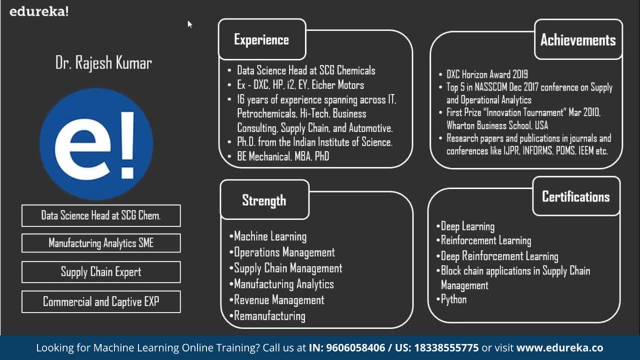 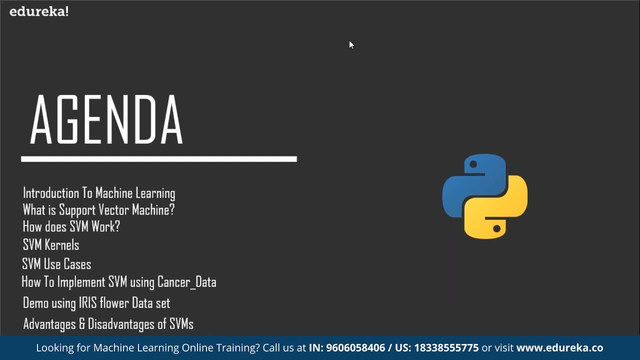 and I have also have got several research papers and publications in different journals. This is the agenda for today, So we will be first quickly going through an introduction on machine learning. We will talk about what are support vector machines and how does it work. 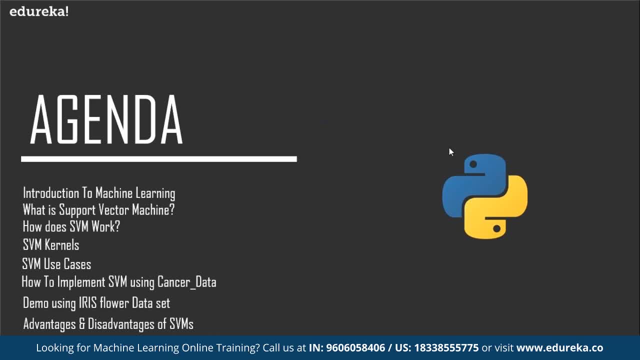 We will talk about something called kernels, which is very important to SVMs, and we will talk about why they are needed and we will go through some of the use cases where SVM is used. We will look at two examples here: hands-on and then, of course, towards the end. 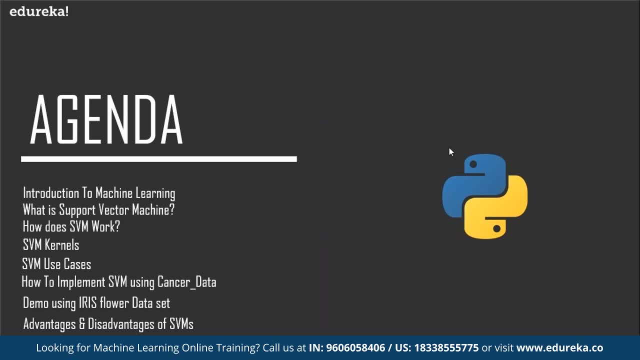 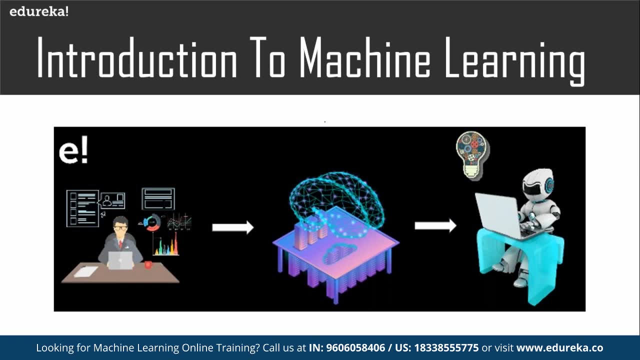 of the session We will be talking about what are the advantages and disadvantages of SVM. Let's talk about machine learning. machine learning is actually a subset of artificial intelligence. So when we talk of artificial intelligence- right as you can see that the phrase is made up- 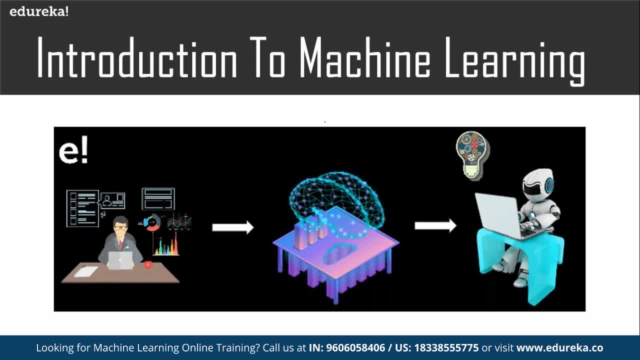 of two words: artificial and intelligence. intelligence generally is associated with what human beings can do, right So, which is basically be able to understand Both spoken as well as written language. you know, we are able to learn from our history, historical experiences, We are able to make decisions, and so on. 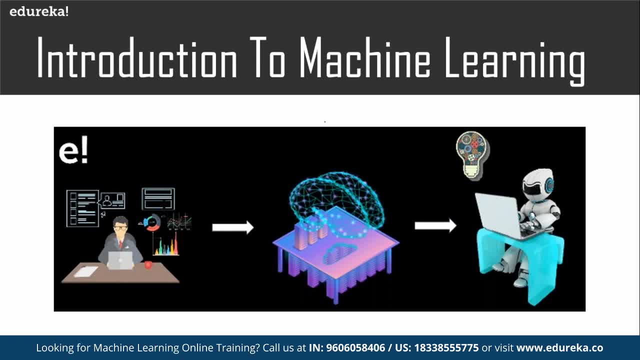 and a lot of creative stuff as well, And so then, obviously, artificial intelligence is about how we can make machines to do some of these things that generally human beings can do right, And, as we said, machine learning is a subset of artificial intelligence. We talked about learning from historical experiences. 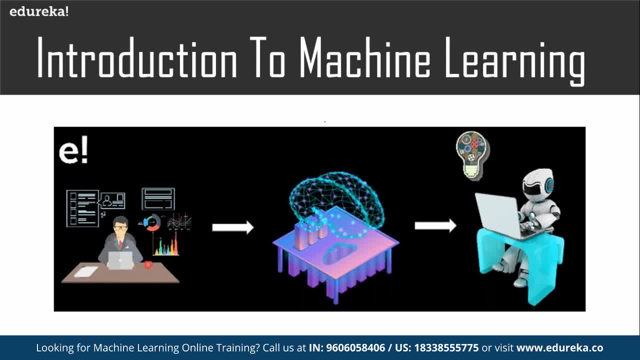 and therefore, if we try to impart this capability to a machine, how can a machine learn from historical information? Then that is what is called as machine learning. Let's take a couple of examples here. right, So I'm sure you know we can differentiate if we are given picture of a cat. 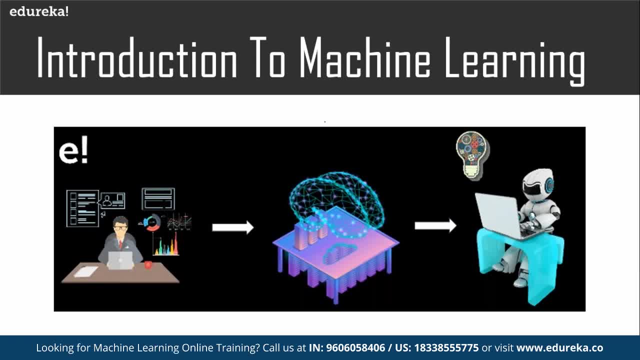 or a dog. right, We can say which one is a cat or which one is a dog, But how about a machine? How can it recognize whether a picture is of cat or is of dog? So therefore, if we are able to build an algorithm, 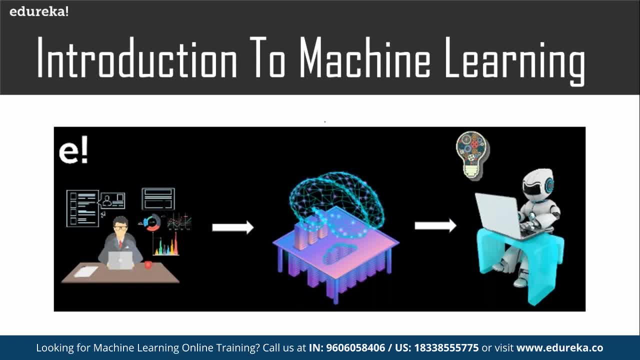 which can learn from, say, several such photographs which we have already labeled it. you know that this particular photograph is of cat, This one is of dog, and we give the machine or the algorithm several such examples and it is able to learn, Learn from that. 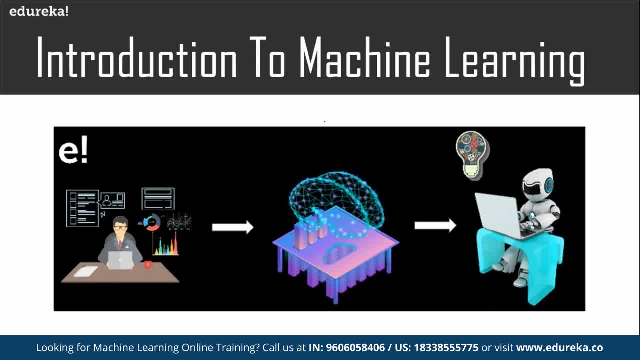 Then we call that machine learning right. So we give it a new photograph of a cat or dog and then, based on its historical learning from previous photographs, It can now classify the new photograph into whether it is a cat or a dog. So that is just, you know. 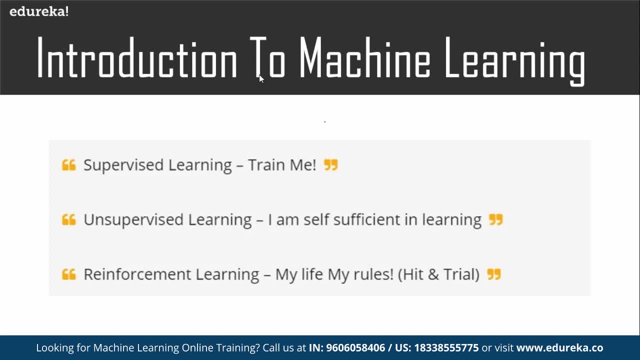 one of the examples of machine learning. machine learning is of several types. right, There is supervised learning, which is essentially that you have Labeled data. labeled data means that you have already classified the historical information, or basically that which sample belongs to which class. 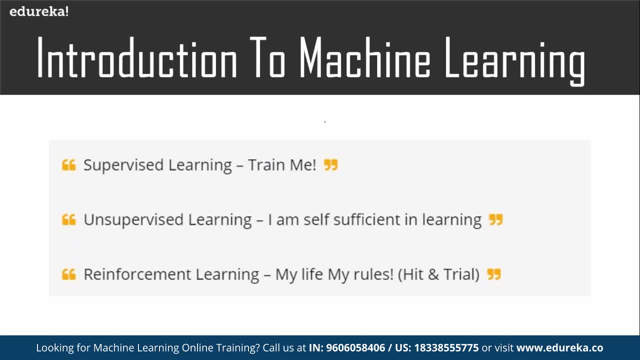 So, for example, a couple of sample of images may belong to cat, or a couple of samples of images may belong to a dog, So that labeled information is already available. So that is called as supervised learning, where you are telling the machine machine or telling the algorithm what to learn. 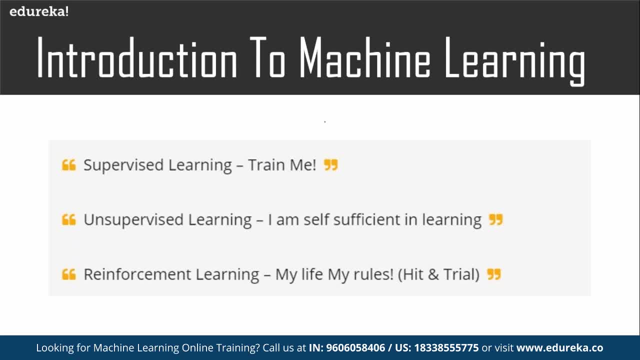 So you are telling it that there are certain photographs that it has to learn as a cat and certain photographs that it you have to learn as a dog. So that is called as supervised learning. Now, what is unsupervised learning? typically, when we have a situation, 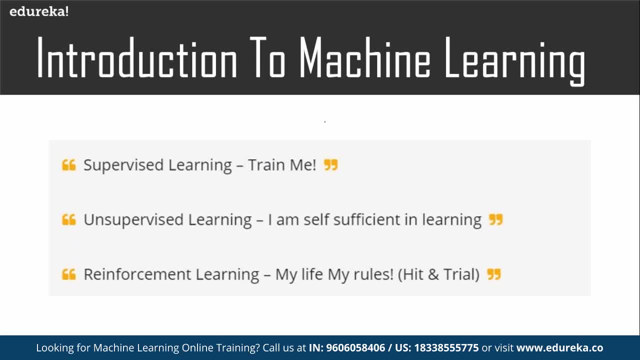 where we don't know about the data much in terms of being able to label it right, like, for example, we have a set of customers and we know about, let's say, the age, sex, the demographic information about where they stay and what kind of you know products. 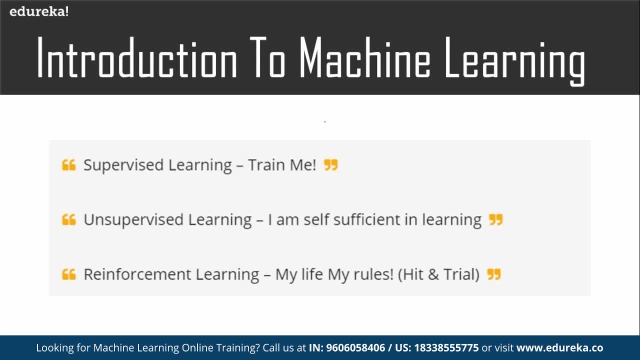 they have been buying Etc, But we don't know anything else right and we would like to find out. you know some interesting classes of these customers, Like, for example: are there specific classes which buy a particular product more or they stay in a particular area? 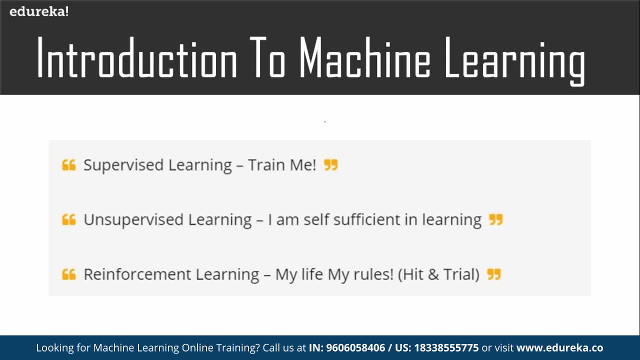 and are interested in a certain kind of product and so on, then that kind of exploration can be done using unsupervised learning. So here essentially we do not tell the machine or tell the algorithm that this is the class of a particular customer or this is a class of a particular sample. 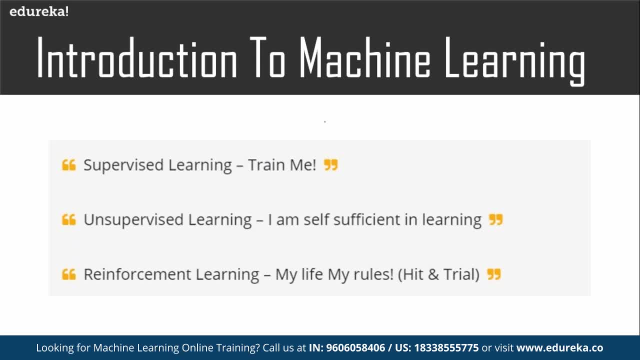 We let the algorithm or we let the machine learn about that by itself, And that's why it's called unsupervised. And then there is a third kind of learning, which is called as reinforcement learning, which is basically as the word reinforcement means. 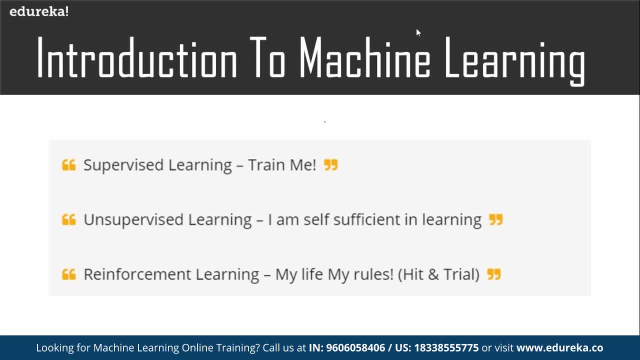 right. essentially, you are trying to learn from your experience that, whether you are moving towards your target or goal or not- like, for example, let's say, you are trying to train a dog to sit right, and every time you say sit, and the dog sits down, and you try to reinforce that behavior by providing it. 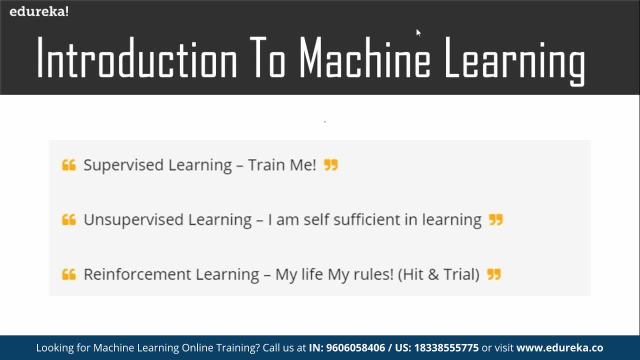 Maybe let's say a biscuit or something like that, And then when it when you say sit, and it doesn't sit and you don't provide a biscuit, it knows that it doesn't get a biscuit when it does not obey the command to sit down. 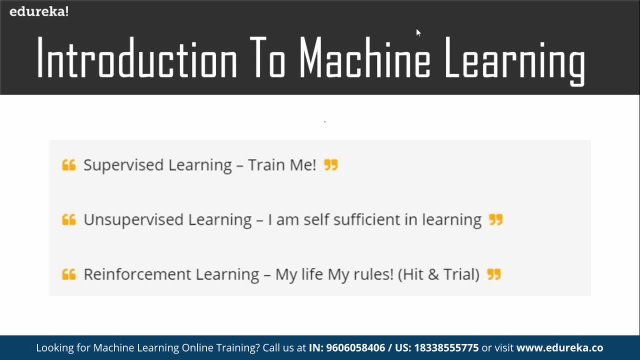 So this is like a reward and penalty kind of scenario, where it gets a reward if it follows or the target or the goal and is penalized by not getting the biscuit if it doesn't follow the command or obey the command. So that is called reinforcement. 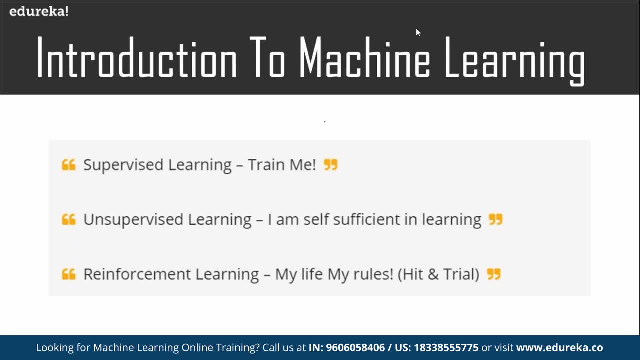 And this is what we also use for machines like- especially if you are wanting an algorithm or a machine to learn how to play chess, but let's say how to play the game go right, or any other sort of such scenarios- essentially, you would like to reward the machine. 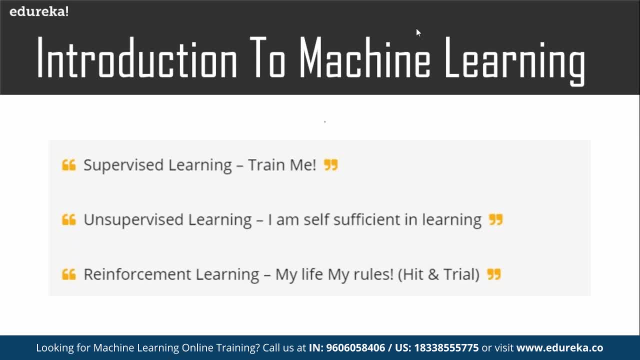 or algorithm every time it is moving towards the goal of winning right, and you would penalize it every time it is moving away from the goal or the target or winning, and this is called as reinforcement learning, which has become quite important These days as well. just to give an example in one: 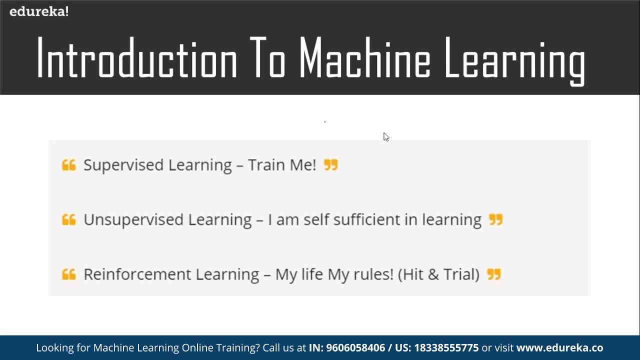 of my projects. we use reinforcement learning for adaptive pricing, which is, like you know. you would have priced your product, So basically you would have kept prices, for for what price each of these products will send in the sell in the market and based on whether the product is actually selling more. 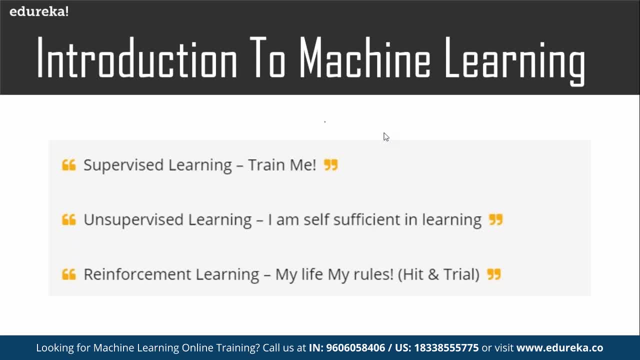 or not, or you are left with a lot of inventory. You can let the machine or the algorithm learn As the actual sales is taking place, and that is what will help it to adapt, to change the prices on its own, you know, by either increasing it, decreasing it. 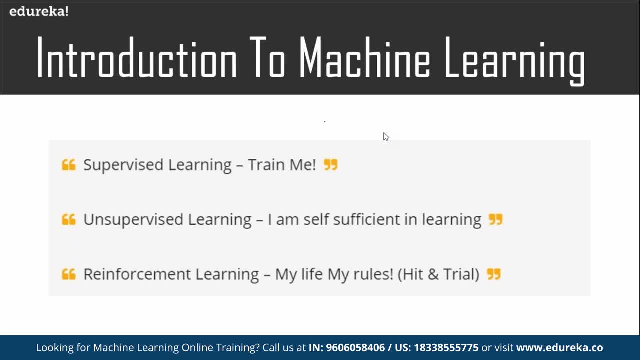 so that the total revenue or the profits can be maximized. This is another sort of a real world example, you know which I have worked on, you know, using reinforcement learning. Okay, So we have talked about the different kinds of machine learning. 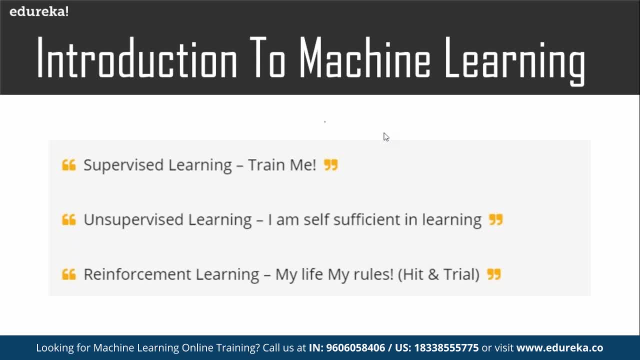 There are several kinds of of algorithms available to do machine learning and we talked about the categories, but the names of some of these are from simple regression models to logistic regression, which can classify. you have support vector machines, You have neural networks. You have several different machine learning algorithms. 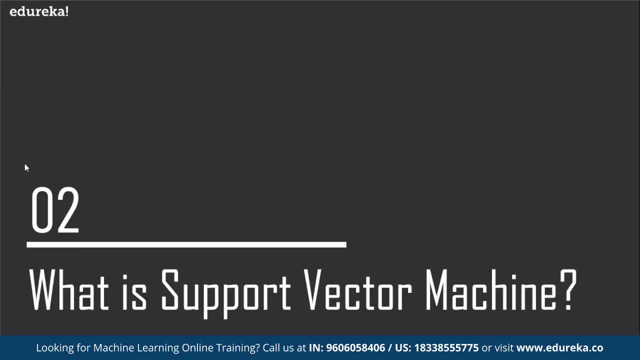 Okay, So now we come to the topic of support vector machine. We have several machine learning algorithms, as we talked about, So why do we really need support vector machines, right, or what is really the need for it? Let's say that we know, that you know. 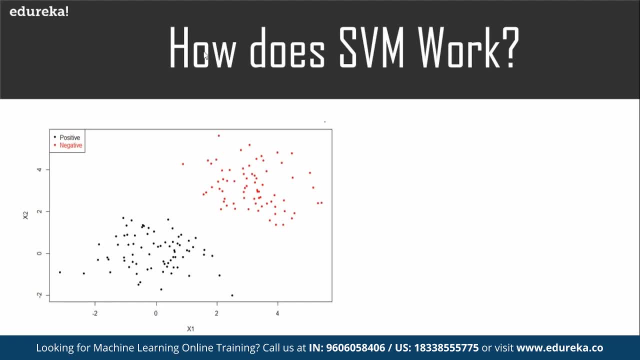 whenever we use machine learning algorithms right to do a particular task, like, for example, here you on the screen. You can see some data points here on a two-dimension: x1 and x2.. Some of which are marked as point as red points, and some of which are marked as as as black points. 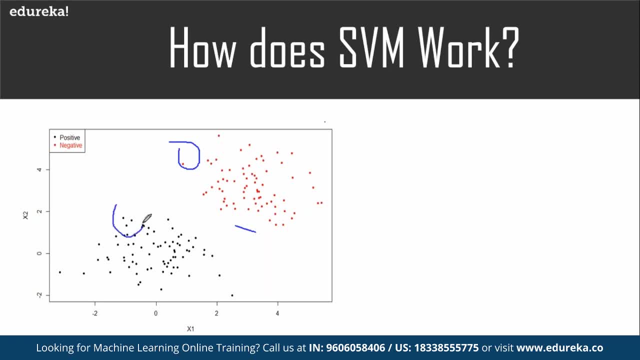 Okay, so you can see the red points here and you can see the black points here. now, typically, what happens is that when you use machine learning algorithms like regression, you may use whatever right. you may use a logistic regression, For example, in this case, to classify this. whether it is 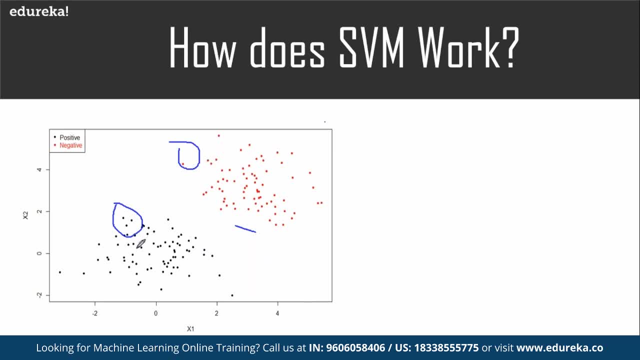 a red point or it is a black point, And all of these machine learning algorithms, they suffer from what we call as bias and variance. right, which is basically. bias is how far from the true classification You are generally, and variance is how much? how much do you vary? 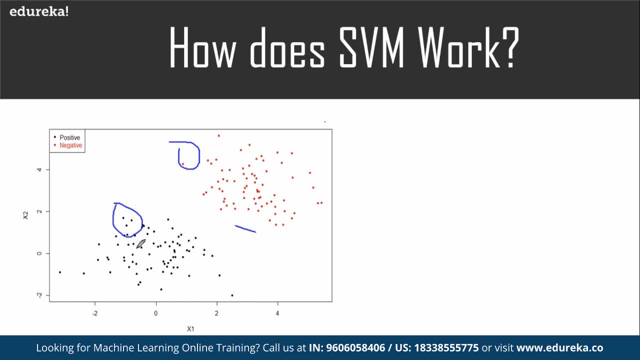 or what is a variance around your prediction? typically the bias and variance they are. they are sort of opposite to each other. So if you try to reduce your bias of prediction, generally the variance goes up and vice versa. So if your algorithm does very well on training data, 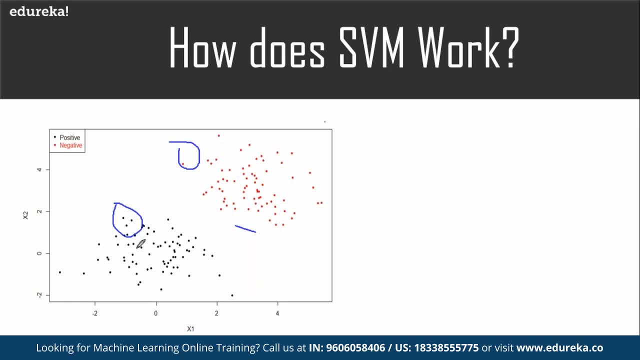 so let's talk about training and test data, right? So you know that we talked about how machine learning algorithms can learn. on historical information, right, where you have already provided labeled data. labeled data, We meant, you know, we already said like, for example: 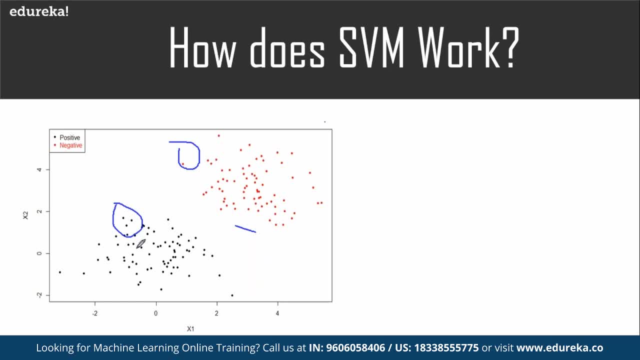 which of the images was cat and which of the images was dog, right and the that data is called as some off. So basically you divide that data set into two parts. So one part is called the training data, on which the algorithm actually learns, and then you test out the model on the remaining part of the data. 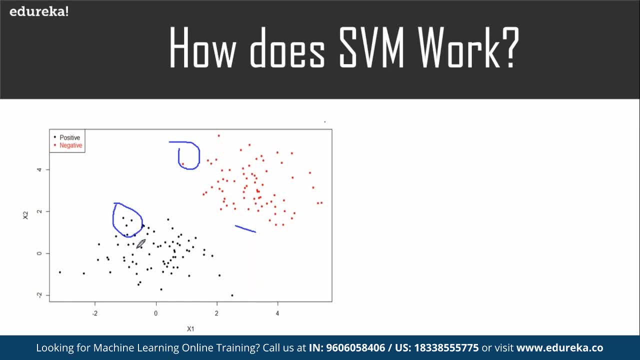 which is called as the test data set, and you try to check. you know what is, how much is the accuracy of your model? Most of the time what happens is that we build a very nice sort of model and it does very well on the training data set, right? 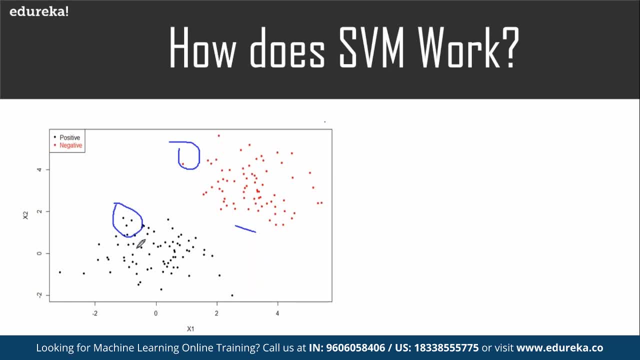 But when it comes to test data set it doesn't do that well and actually the the taste of the pudding is in the eating right. So even if my accuracy on the training data set was in the high 90s, but my if the accuracy on the on the test data is not very good, 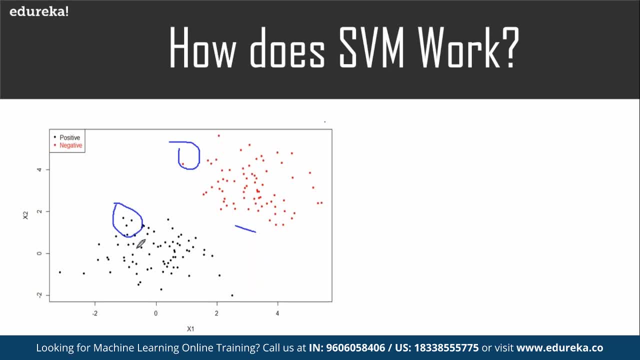 Then my model is not very useful, right, is not very usable. So that is the reason why you know, support vector machines actually come in there and they are. they are much more helpful there because they can help to generalize the models much better. when we say generalize, what we mean is basically the model may not work. 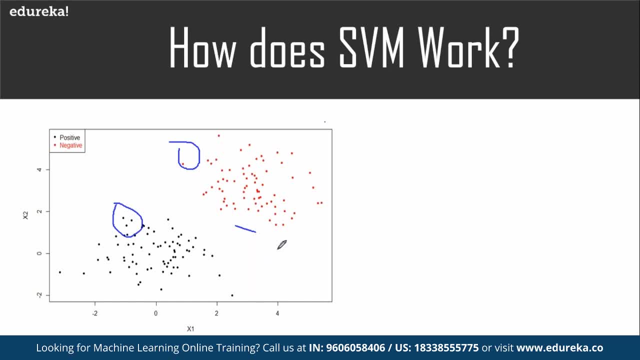 that fine or the accuracy may not be that high on the training data set, but the accuracy is quite good on the other test data set generally. So that's sort of the motivation on why we need to learn support vector machines. Now we will talk about how SVM works. as you can see, 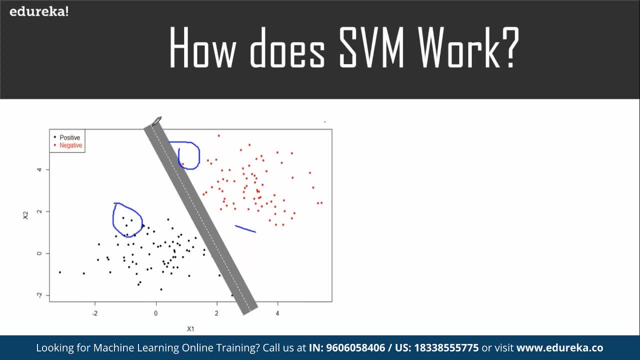 you know, we can create a hyperplane. a hyperplane is basically a plane in n dimensions, right? So here, actually, you can see that there are two dimensions here, X 1 and X 2, and there can always be a third dimension which you can see in 3D plots, right? 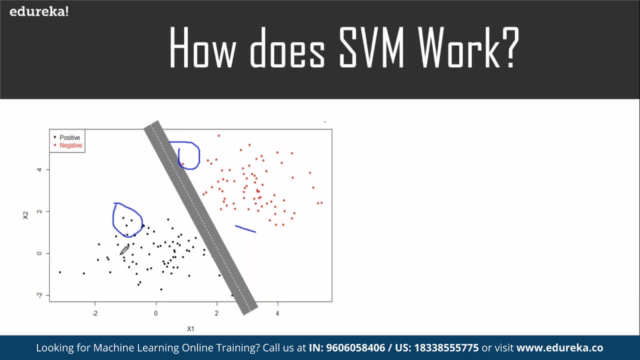 But you can also have a lot of other dimensions which is difficult to visualize. obviously as human beings We cannot visualize, but a computer can do calculations of distances etc in that high sort of dimension as well. So that n dimension plane is called a hyperplane, as you can see. 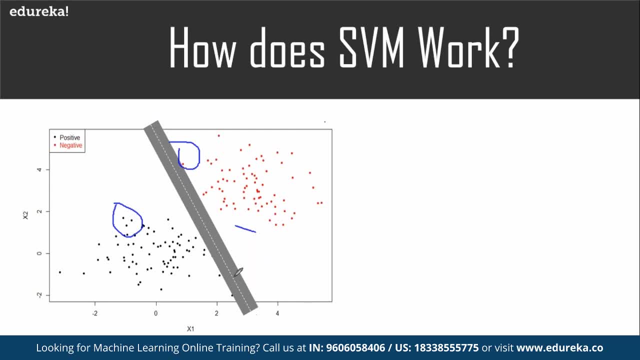 We have tried to draw this hyperplane here Which kind of classifies these two data sets here and now. there can be several such lines that can be drawn, So you can see there is another line here and then another line here. So, as you can see, this line probably is the one. 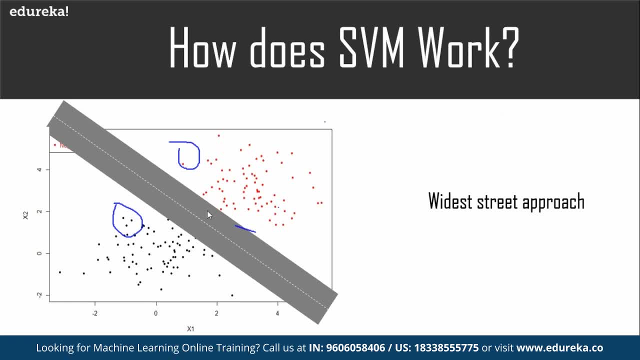 with the widest margin between the two data sets. So this particular data point here and maybe another one Here, right, But this, if you look at this hyperplane, for this hyperplane, probably the nearest points are that it is touching is this one. 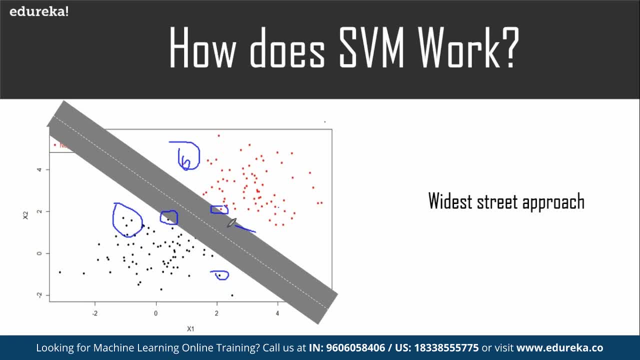 right And maybe here the red and the black one. So the widest Road or the widest treat that is possible between these two data sets is using the one, the hyperplane that you can see right now, The, rather than the hyperplanes that you saw earlier. 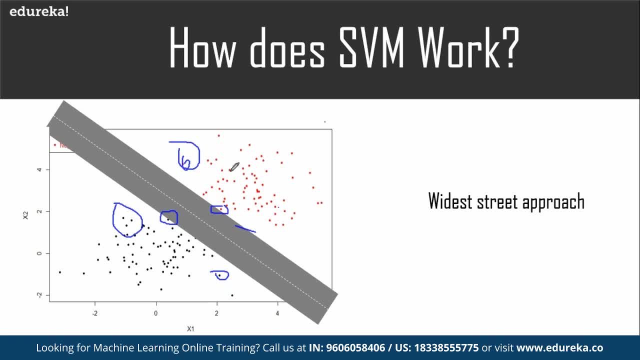 and this is what SVM tries to do- actually tries to build a hyperplane that separates the classes or like, for example, the two data sets here, with the maximum width of, or the widest Street that is possible, As you can see in this particular case, and these two data points which you saw here, the ones which are lying on the 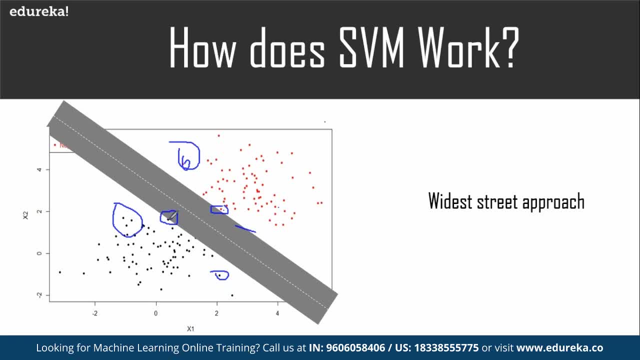 Edge of this particular Street. they are called as support vectors because we know that every point is like a vector in the n-dimensional space, right or example. in this case It's a two-dimensional space. So so, basically, if you drop or sort of perpendicular from from these two data, data points onto the hyperplane, 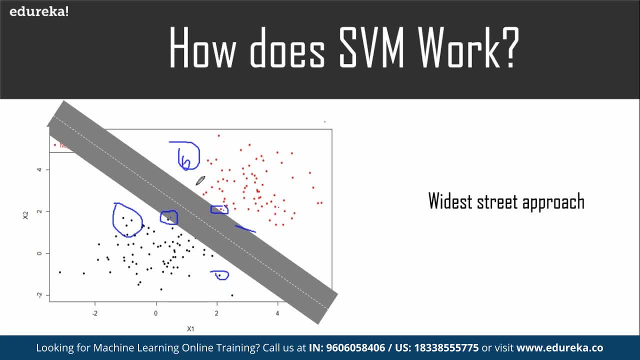 then that the, the summation of that will give you the, the width of this particular Street, and these points are called as support vectors. And if you remove these two points, what happens is the solution changes and, and, and. therefore, how can we identify the support vectors? 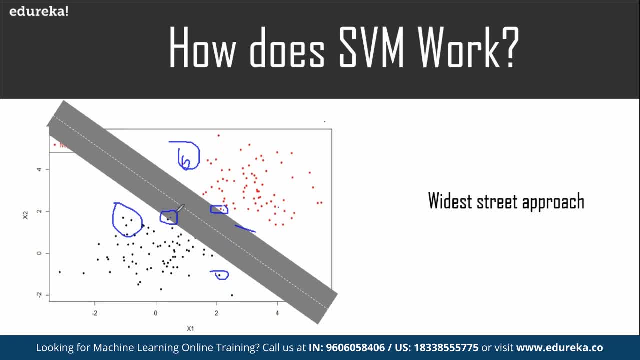 Well, if on removal of these data points, the support, the solution doesn't change, then obviously those points are not supported. Let us, let's go ahead and let's move on to. okay, Let me just remove these Drawings here that I made, and just to summarize what we meant by: how does SVM work? 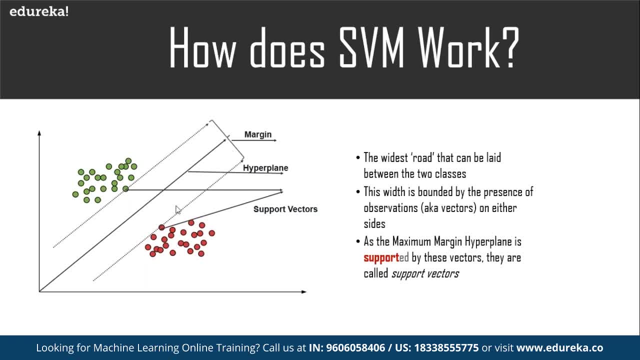 So we have to create like the widest road that can be laid between these two classes. It is bounded by presence of observations which we call as support vectors, And this is the hyperplane in the middle which has got the maximum margin supported by these vectors called support vectors. 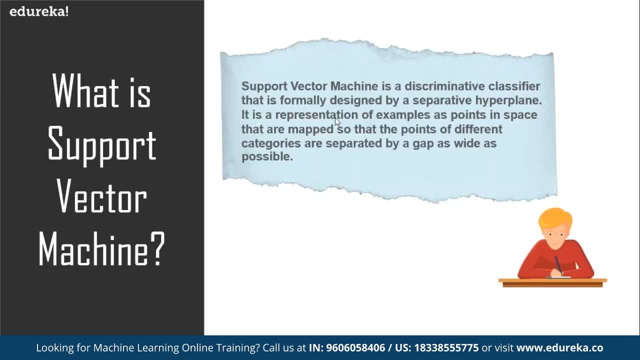 So coming back now to the definition of what is support vector machine, So support vector machine is a discriminative classifier that is formally designed by a separative hyperplane, which we just saw, and it is representation of a of points in space that are mapped. 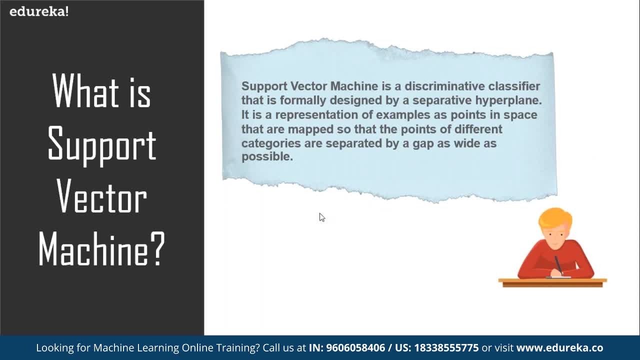 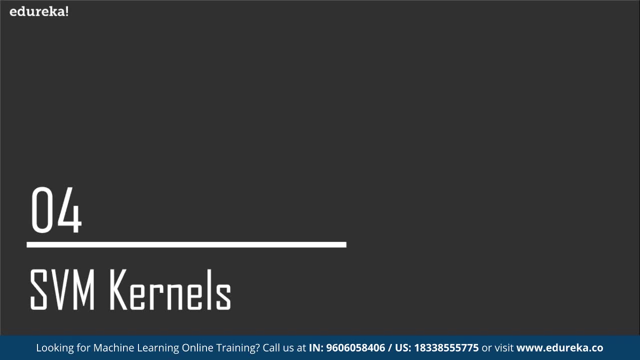 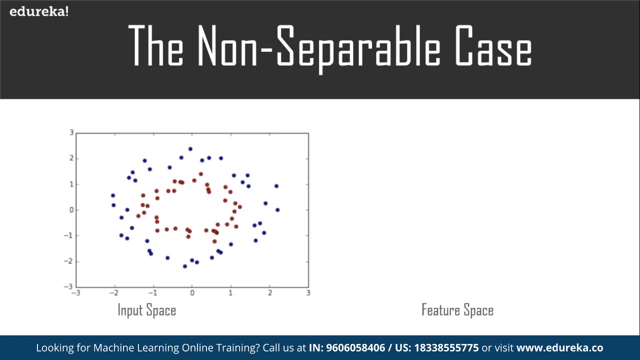 So that the points of different categories are separated by a gap as wide as possible, which we just saw. So we now come to a very important part of support vector machines which is called support vector machine kernels. So we had earlier looked at an example where it was very easy to classify. 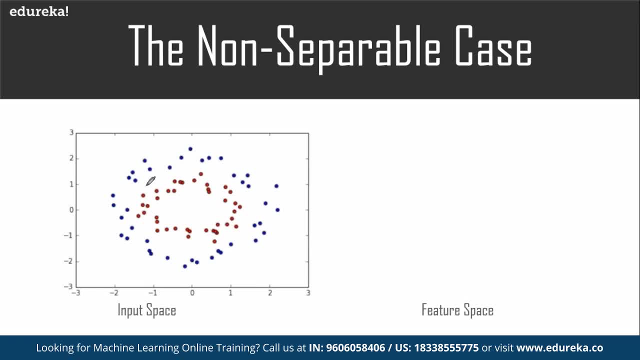 It was quite easy to classify in that case. But here you see that the red and the blue dots. They cannot be classified by a line, right? So you have this data: points in the center which are red and the ones which are surrounding it. 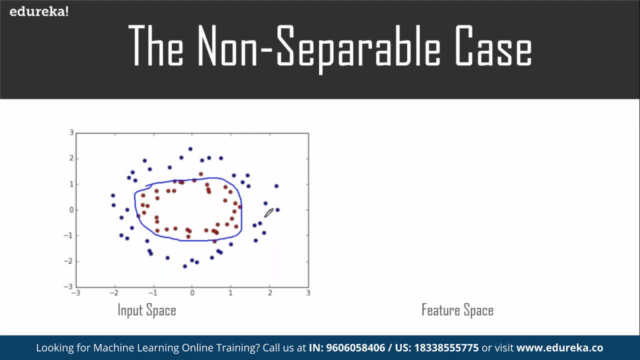 which are blue in color. Now, this is a non-separable case. How can support SVM work in this particular case? So what happens is, generally we use what is known as a kernel trick, and I will talk a little bit about kernel trick. 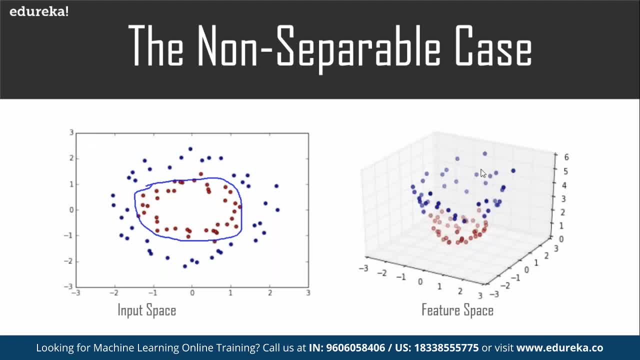 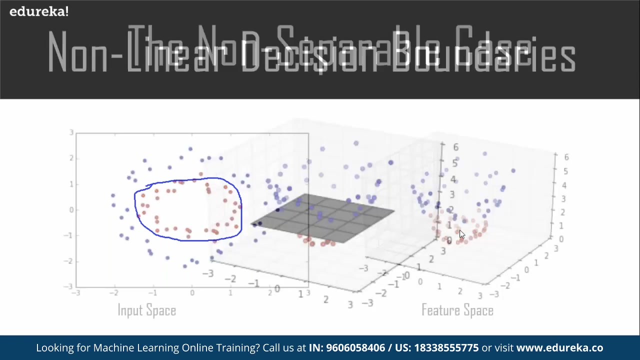 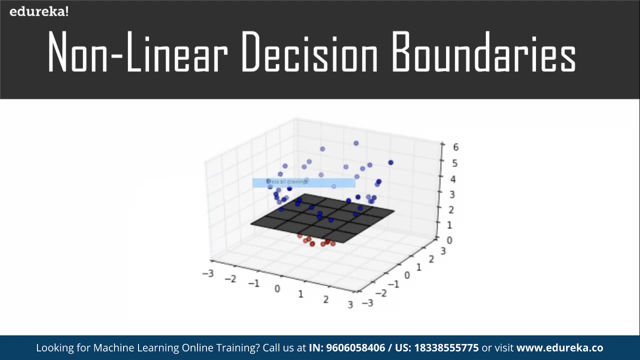 So essentially, what happens in a kernel trick is that you map this input data space, which was in a two-dimension, To a higher dimension space, which we call as feature space. So you transform all of these points and, as you can see, it becomes quite easy to. it becomes quite easy to to segregate these two data points. 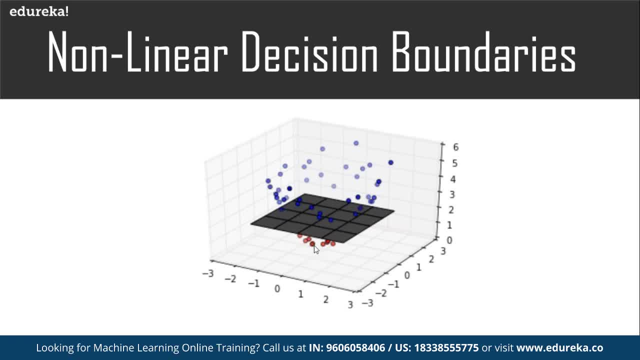 as you can see this parabola here you have the red dots below and the blue dots above. So we have just transformed the input space into a three-dimensional feature space And now you can draw a hyperplane which you can see, which has been made here in between. 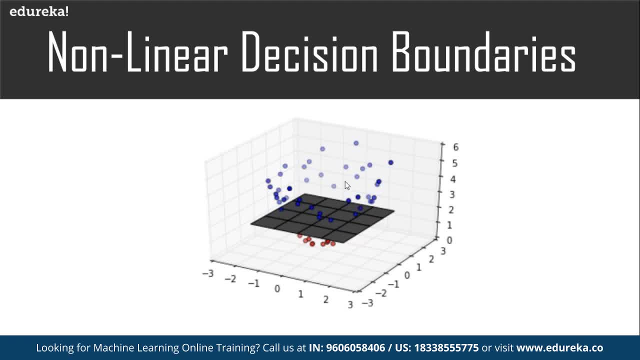 which can separate these two classes. So generally what happens is, if you are able to map the input space into a higher dimensional feature space, it becomes easy to create a hyperplane which can which can classify thus the the classes of information or the data points that we have now. it generally is very tricky to 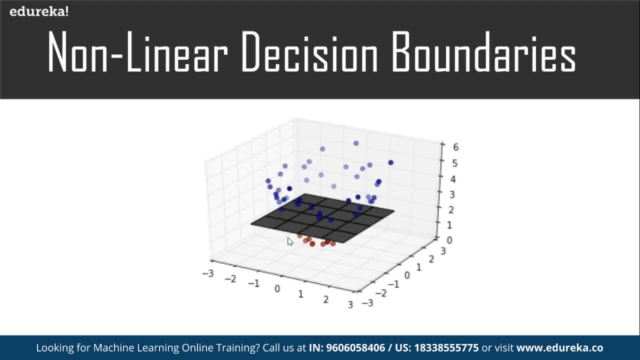 map all of the input data points into, into the higher dimension, and it requires a lot of calculation and therefore it may take a lot of time, and that is where the kernel trick comes into picture. So a kernel is a function that helps to map the input space into the higher. 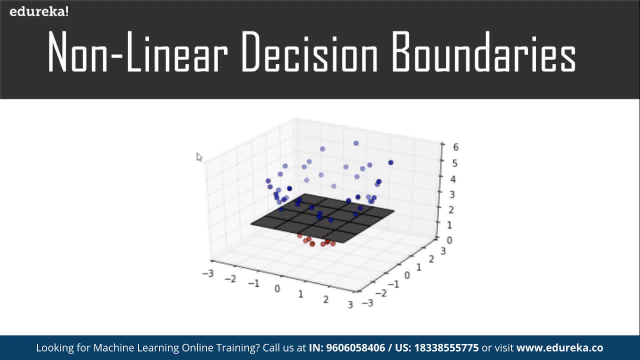 dimensional space or come or compute the hyper plane without being able to move all of the input space data points into the higher dimension space. So it only looks at like, for example, the closest points we have seen right. How can we calculate the similarity? 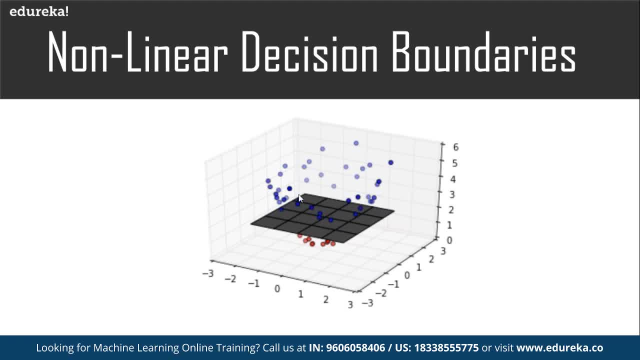 between the higher dimensional space and the higher dimensional space, Between the data points, these red, for example, the red data points and the blue data points. How can we calculate the similarity? and later on, when you read about the details, you will find that this similarity is called a cosine similarity. So how can we calculate these? 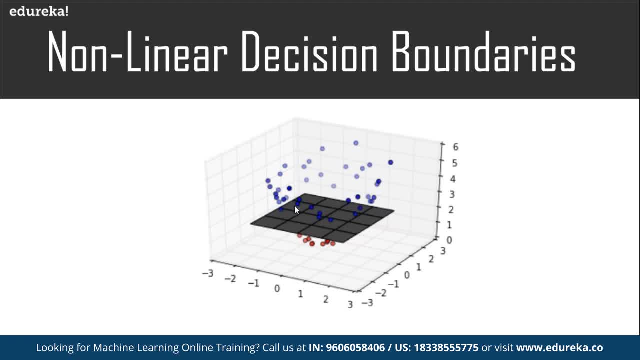 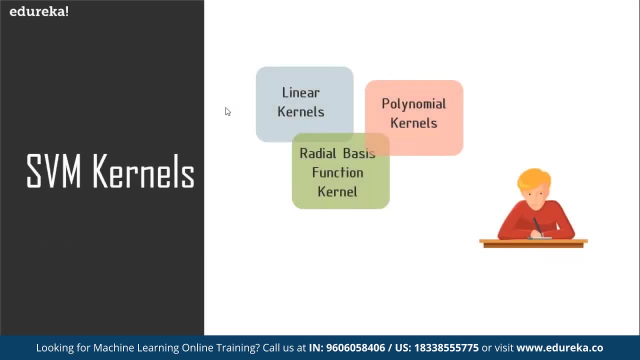 cosine similarities. you know, using the function which is known as a kernel tray, and there are three different kinds of kernels here. One is called as the linear kernel, The other one is called a polynomial kernel and the we have the radial basis function kernel as well. as we move from the radio, from 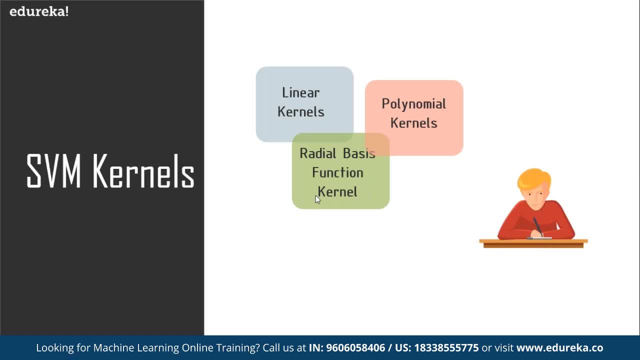 the linear to polynomial to radial basis functions. generally the complexity of the functions increases. So linear kernel obviously has the lowest complexity and the radial basis function has the highest complexity. right and most of the time for implementation. People use radial basis function because it can help to map the input space into an infinite dimension feature space. 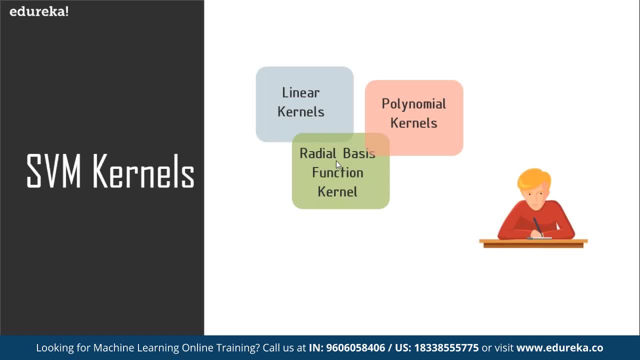 So that is the power of radial basis function. It can actually map any input space into a infinite dimension, you know feature space. That is the reason why it is easy. It becomes easy for the support vector machine using a radial basis function to actually classify. 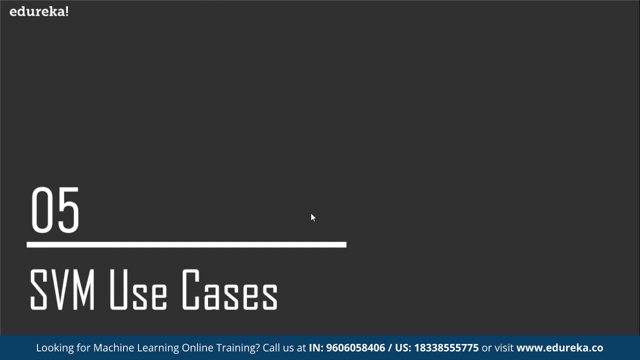 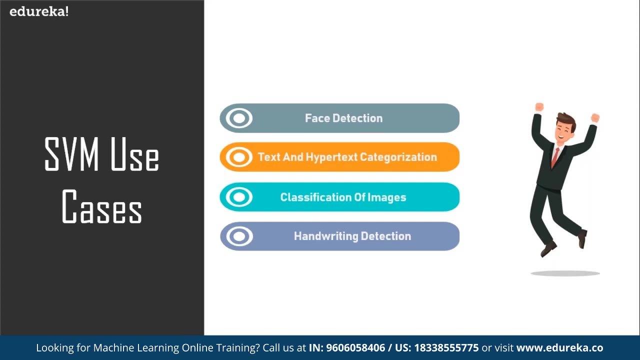 you know data sets. We will talk about now some of the use cases of support vector machine. So support vector machine, as we said, you know they can be used for face detection, Like, for example- you know you are trying to classify, maybe let's say who is who are terrorists and who are not right- or text and hypertext categories. 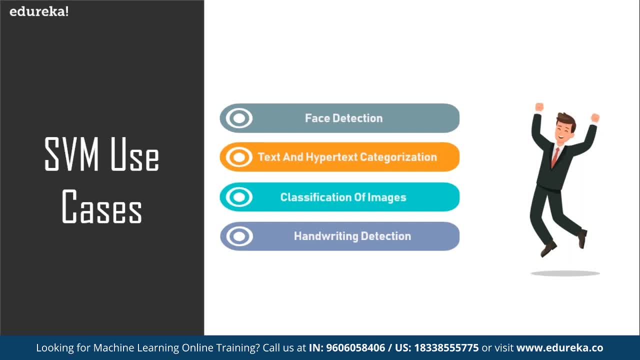 Right or text and hypertext categories, So you can actually, like you can, have the support vector machine be used for face detection, hypertext categorization, classification of images, handwriting detection and so on, and also in the bioinformatics space views that I have used personally. 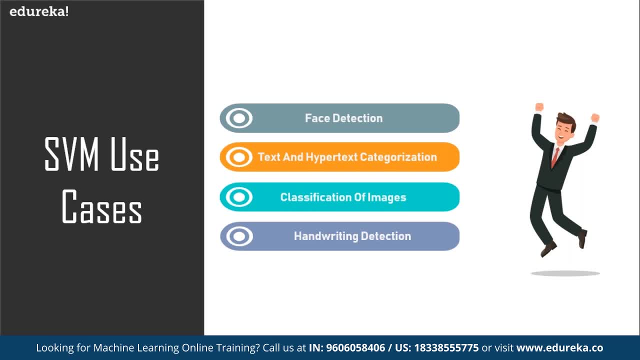 I've used support vector machine in supply chain kind of use cases where we were trying to, you know, predict whether a supply chain risk will happen or supply risk will happen in the future or not. So I've used four of them. They are you know, so we are going to use this one. 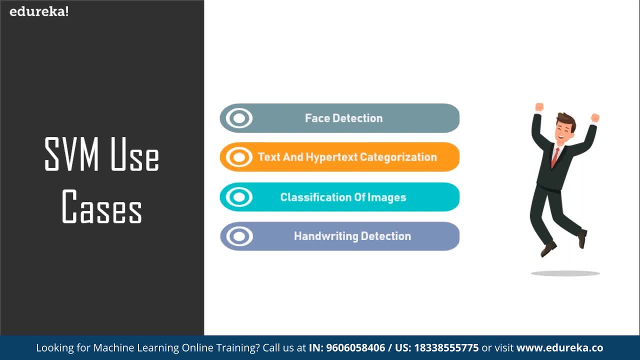 So I've used four of them, support vector machines there. I have also used support vector machines for a particular company where we were trying to classify in the warehouse whether some of the boxes or pallets they are misoriented or they they are, you know, missing. 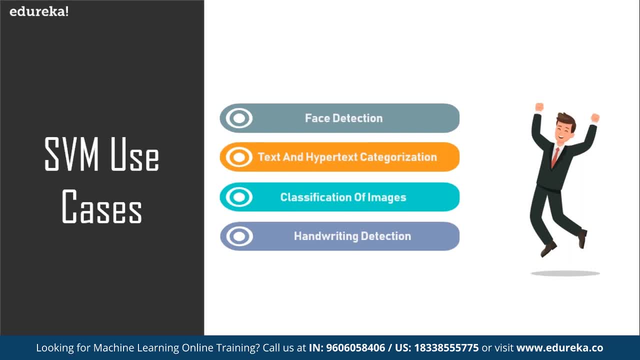 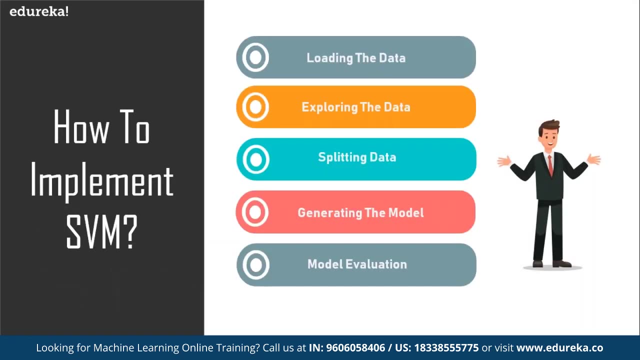 because somebody has stolen it, and so on. So classifying information of inventory into several classes using support vector machines. So these are some examples where SVMs are used and now how to implement SVM right? So essentially, implementing SVM follows similar process, as you know: normal, you know. 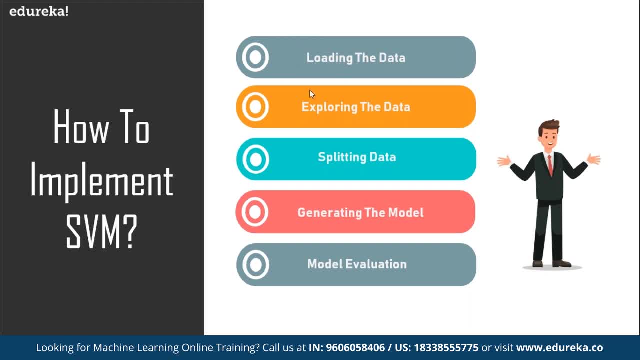 you are implementing any other machine learning algorithm. So basically, you have to load data, You have to explore the data, which is called as exploratory data analysis- You have to split the data into training and test set, and then you have to generate the model. 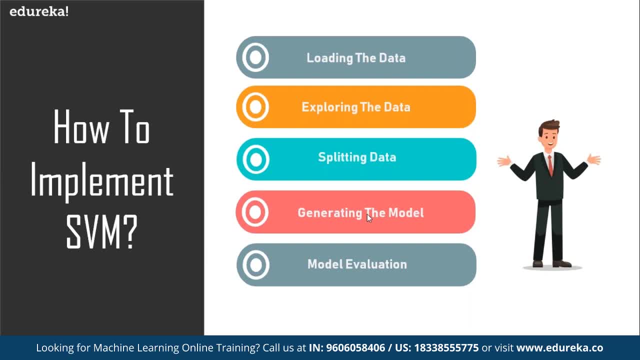 You have to do the hyper parameter tuning to make sure that your model is working well and you get the desired accuracy. and then you have to- obviously for that you have to do a model evaluation to check you know how accurate your model is. So what we will do is: we will quickly get. 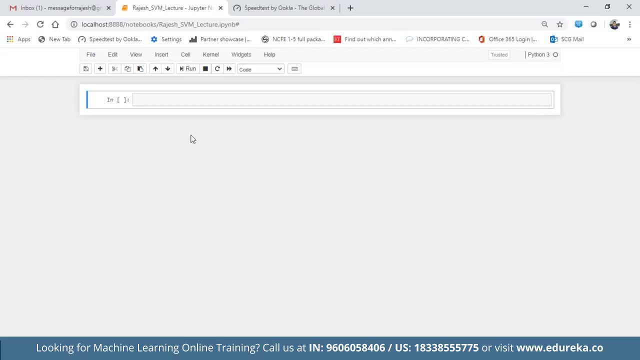 into some hands-on here. So what I have here is essentially a Jupiter notebook which is in stock. It's called on my laptop here and we will first take up a data set which is there as a part of the scikit-learn package itself. 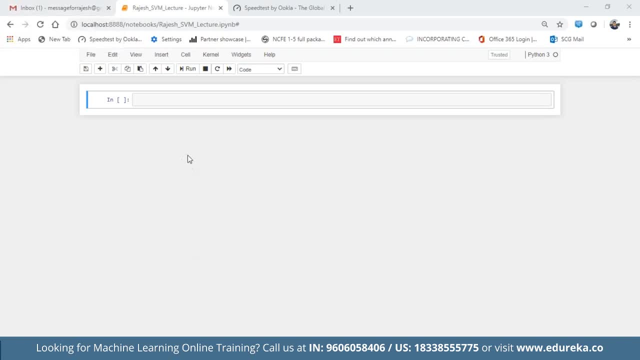 within Jupiter notebooks and it's called and it's data set related to cancer, right? So whether a cancer is malignant or benign, been a malignant means it's bad cancer and benign means it's it's okay, It's a, it's a tumor which doesn't grow, right? 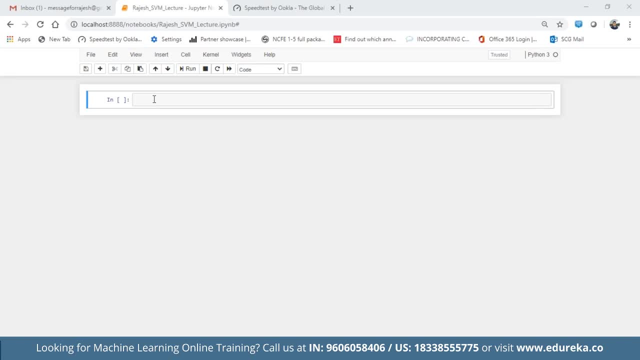 So how, based on information, on tests and on these tumors, how can we classify whether a cancer is malignant or or benign? So that is what we will look at. Okay, so we first we will start by importing the libraries here which are needed for this particular example. 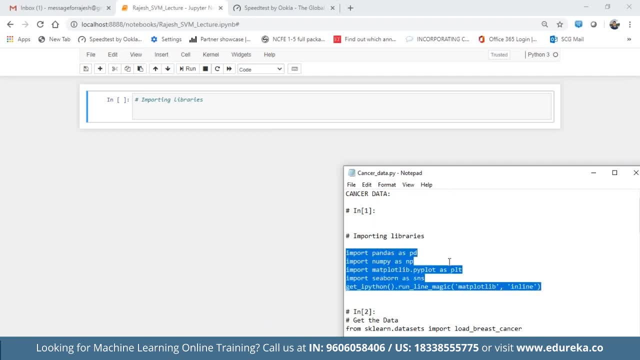 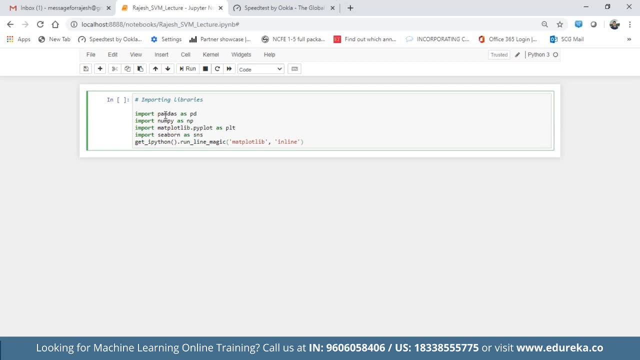 And we know that for machine learning the typical libraries we use right numpy for all of the numeric functions and you know pandas for arrays, for data massaging and so on. matplotlib generally we use for plotting of the data sets and seaborn is another visualization package And essentially the line here: get by ipython here. 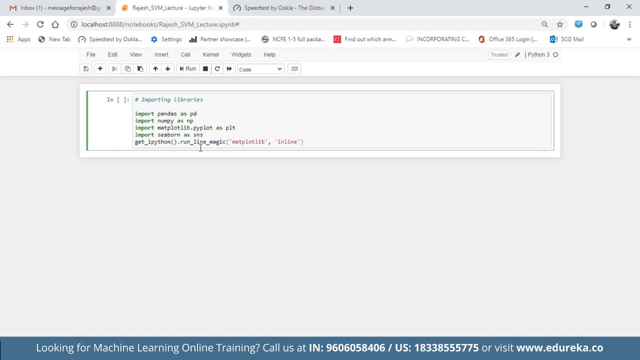 is basically saying that we want to show the matplotlib picture in line in the Jupiter notebook itself instead of creating another sort of tab. So we run this and what it is doing is it is importing all the libraries, and then it has already run, and now we 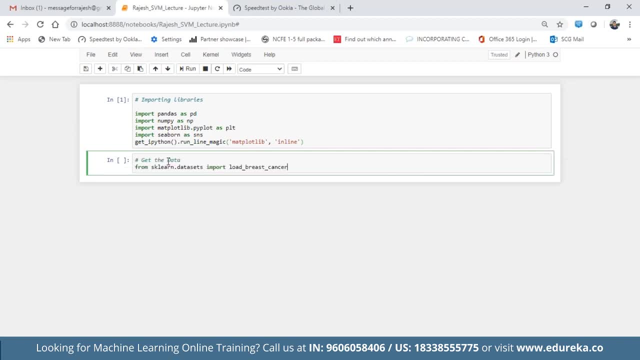 will get the data set right. So we will this data set. We are importing from from SK learn, which is scikit-learn, and we are importing the breast cancer data. So it's it's it's got loaded and now we will what we will do. 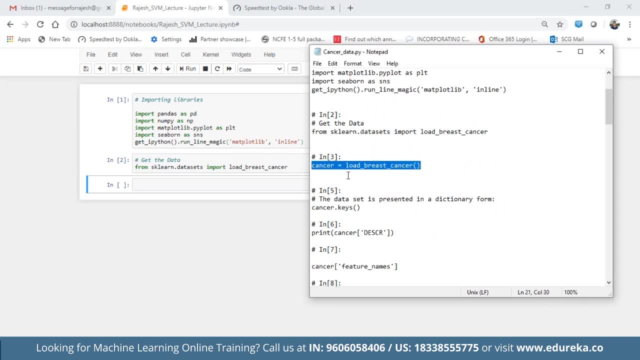 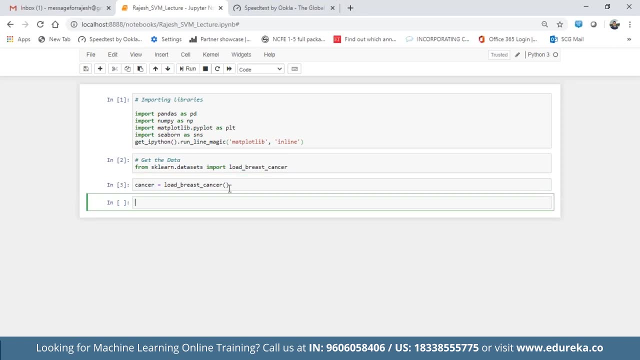 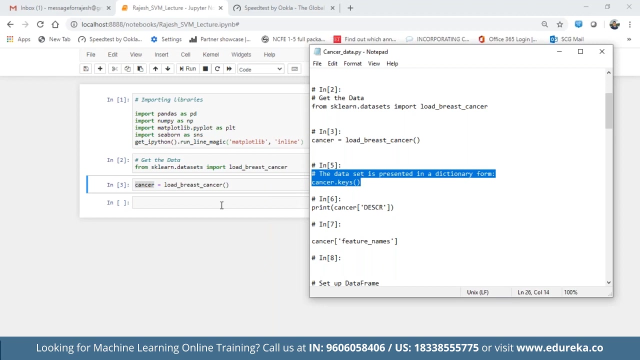 is, we will actually import this data Into this particular variable here called cancer. So the cancer variable here now has all of the data related to the breast cancer And we- now we will look at some of that. What does this data have? right? 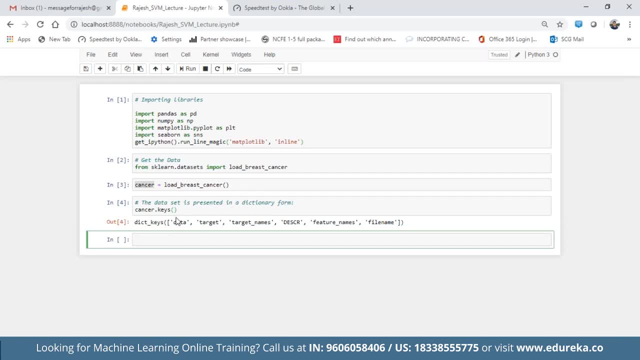 So actually this data set is in a dictionary form, So you have the keys in the cancer data is that we have some data. There is a target variable which is basically telling us whether the data, whether the cancer is malignant or benign, and there are the names of the targets. 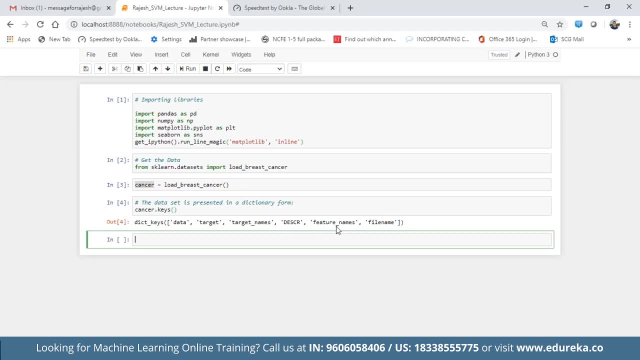 and there is a description of the data itself, the feature names and and file name. So these are the various attributes of this particular cancer data. Actually, let's look at some of it. So let's print the. You can print the description of the data. 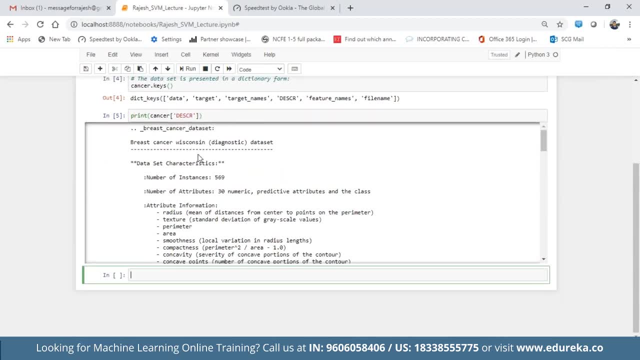 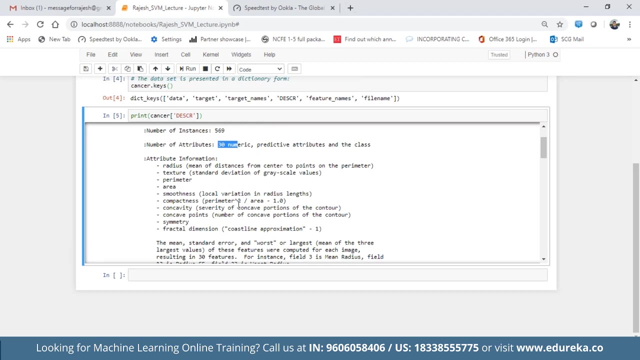 like this using this particular command, and we see that it gives you all of the information related to the data here. So it has about 569 data samples and number of attributes are 30. They are all numeric and you have information like radius, texture, smoothness, compactness and so on. a lot of it. 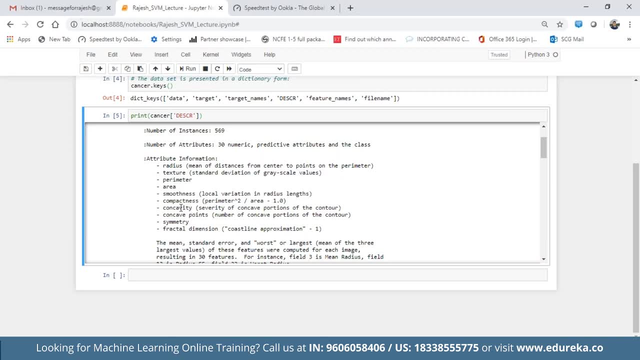 So you can print the description of the data like this, using this particular command, and we see that it gives you all of the information related to the data here. a lot of it is actually related to the medical field, right? So we may not understand it. 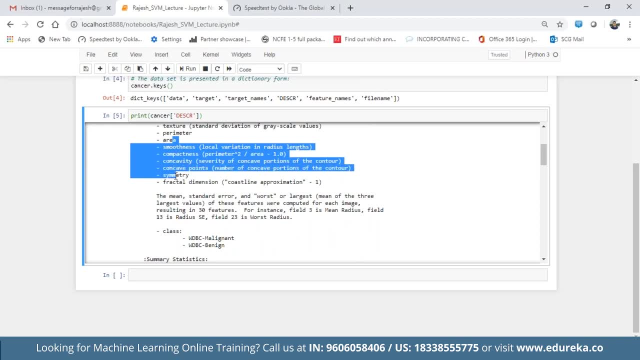 but essentially, what you should understand is that these can help to predict whether a cancer is malignant or benign, and that is what the two classes are here. And then we have some summary statistics related to what is the min and Max of each of these values. 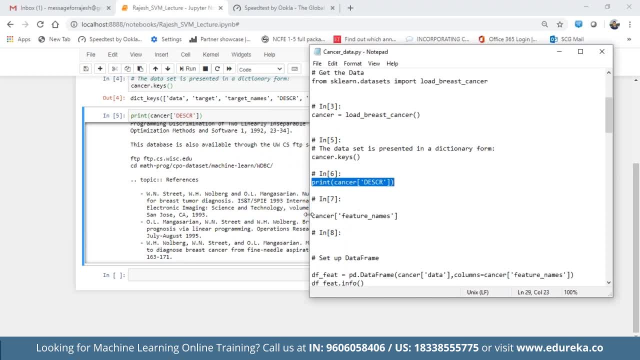 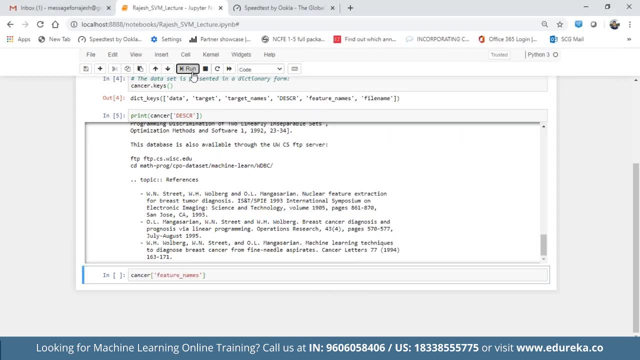 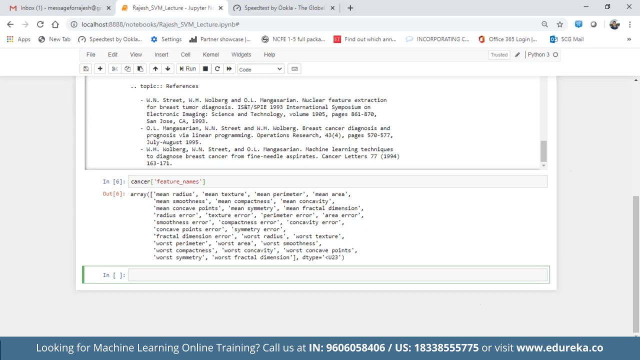 Okay. so now let's quickly look at what are the 30 features, or the feature names, really right? So if we run this, we see that these are the 30 features: the radius, texture, para, mean parameter and so on. now we will set up a data frame. 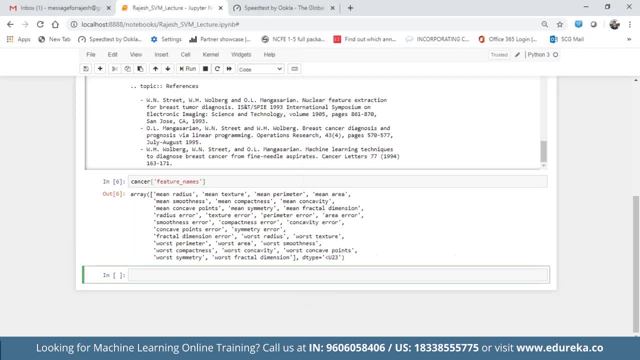 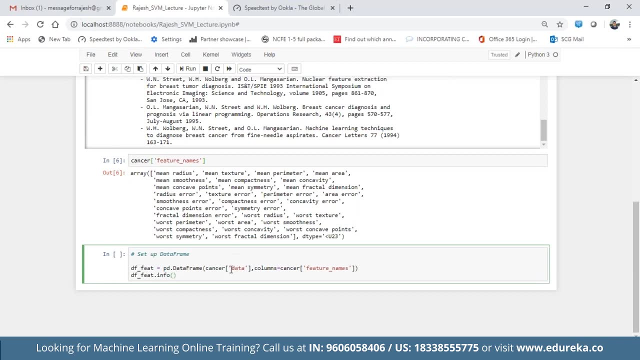 so that we can start doing and building our model. So we create this bandage data frame from this data, So we take the cancer data and the column which respond to this but correspond to these feature names, And then if we look at the information, so you can either use this particular function info. 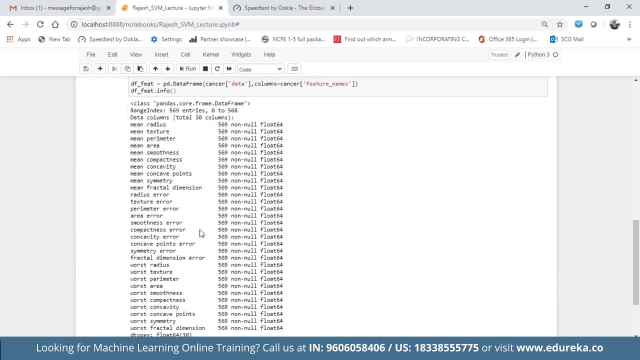 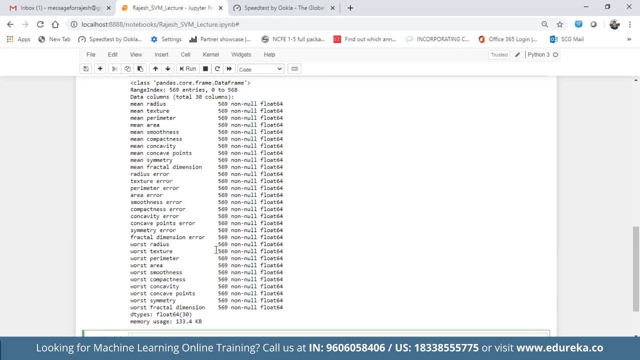 or you can also use describe function to actually look at the summary of the data. So we have all these columns that we talked about. There are 569 samples. There are these 30 columns. All of them are our float values. Okay, 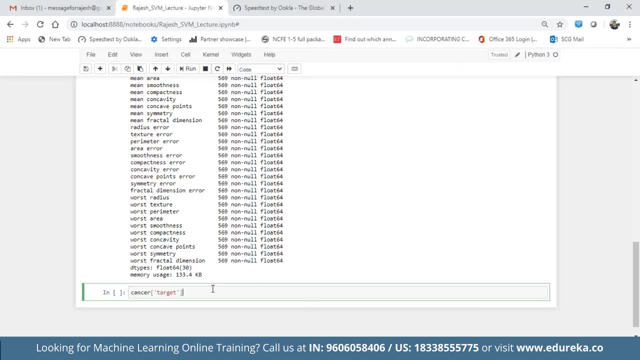 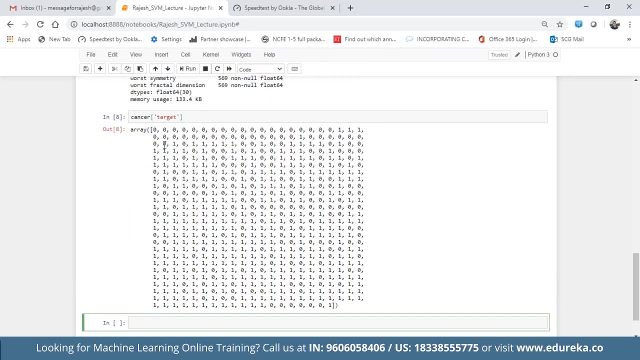 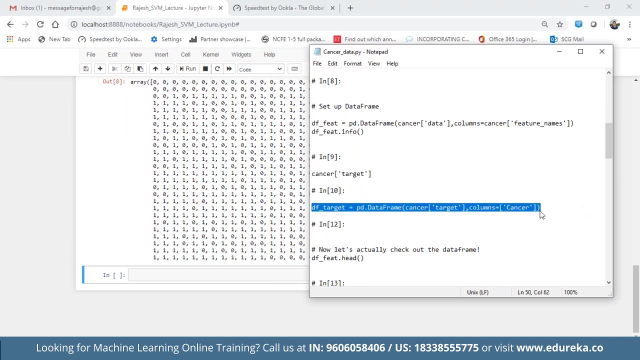 So now we let's look at our target variable, which is the array of zeros and ones. So 0 basically signifies that it is malignant tumor and one signifies that it is a benign tumor. And so now, so we we take the target variable. 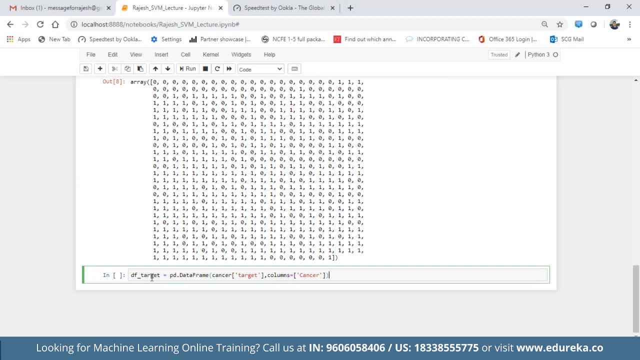 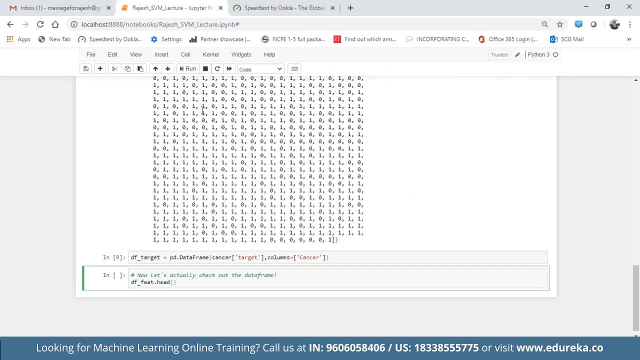 which is whether it is cancerous or not, or malignant or not, in this particular variable here- TF, underscore, target. And then let's check out the data frame Now, once we have built it, so you can see that this is like the top five rows here. 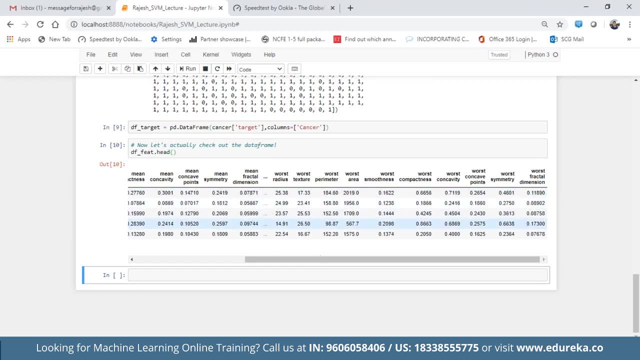 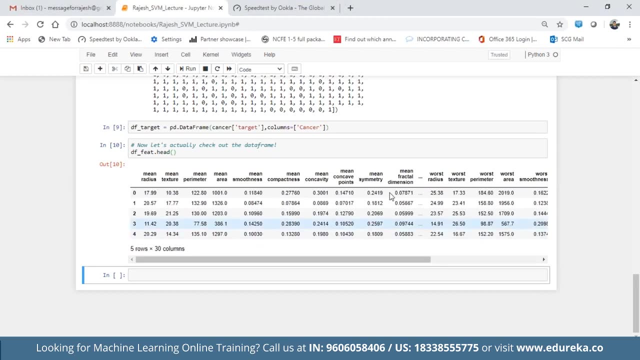 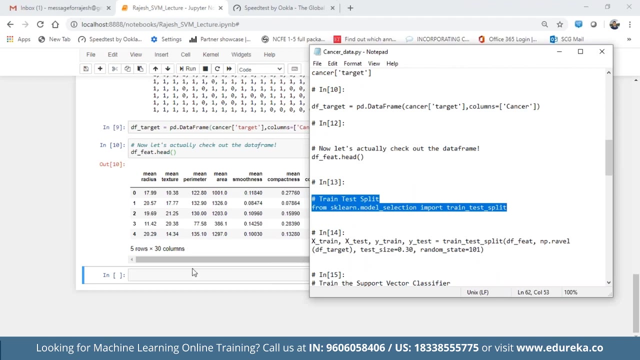 but there are 569 of them, and you can see all of the values related to different features which can help to predict whether this particular cancer is benign or or or malignant. Okay, So now what we will do is, as we talked earlier, we have to divide the data set into two parts. 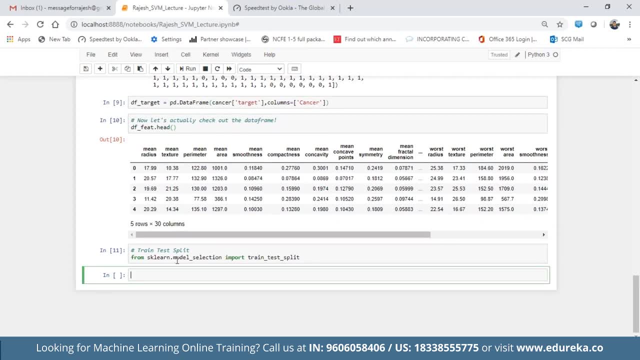 which is training and testing data set. We use the train test split feature of the psychic learn package, which helps us to do this automatically. Now what we do is we: we have to decide how much of the data we have to keep as training and how much of it is test data. and we, here, we are keeping. 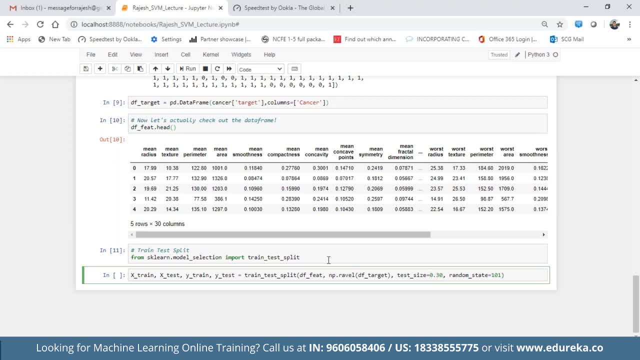 the test data size as 30%, which means that the, the training size is 70% and the random state here 101, just means that we, if you use the same random state, then you should get the same results as me. Otherwise our results may differ if you are trying to code along. 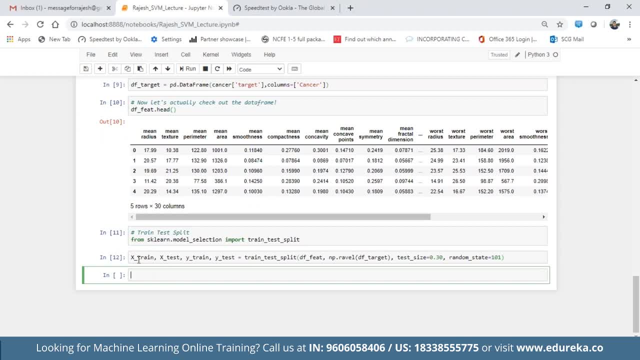 So what we do is we get all of the information into the X train and Y train, which Y train is basically the target, which is basically whether it is malignant or or not, And the test. it also has got the X test and Y test similarly. and now we, what we do is we, we will now do. 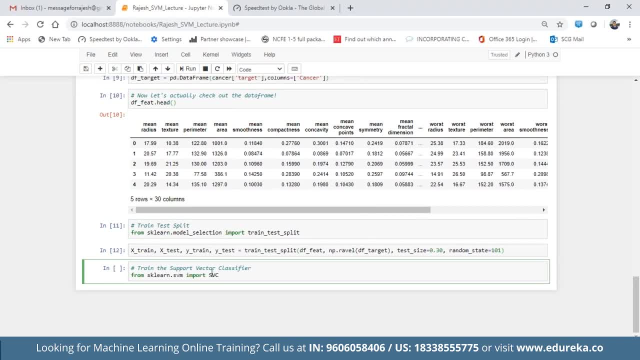 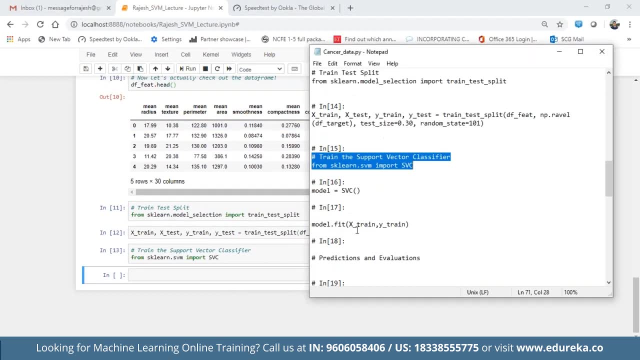 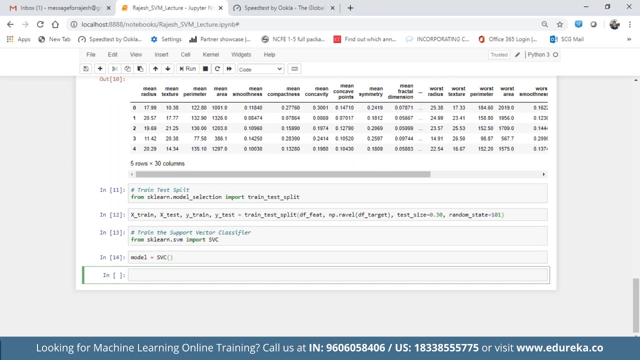 the support vector classification. So for that we import the support vector classification algorithm from psychic learn and we'll go ahead and we'll initialize this into our variable call model. So model here now represents a support vector classification Model and we will now do a fit, basically. 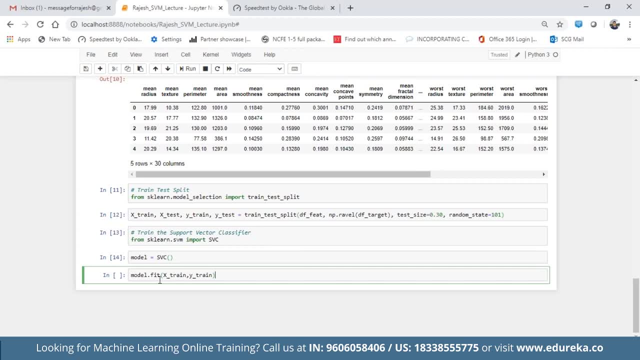 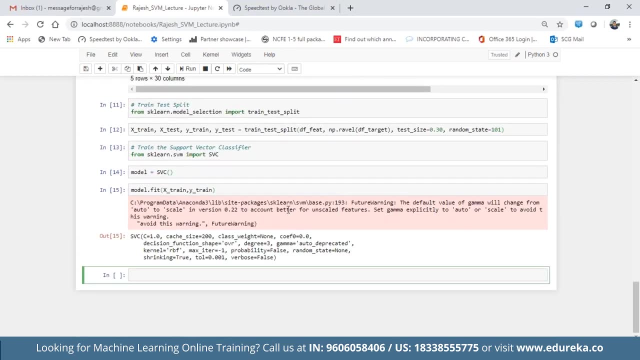 We are training now the model on X train and Y train using this support vector classification. This is just a warning. nothing based on you know version numbers. You will get some warnings but it is not an error here. So the what we see here: there are several hyper parameters. 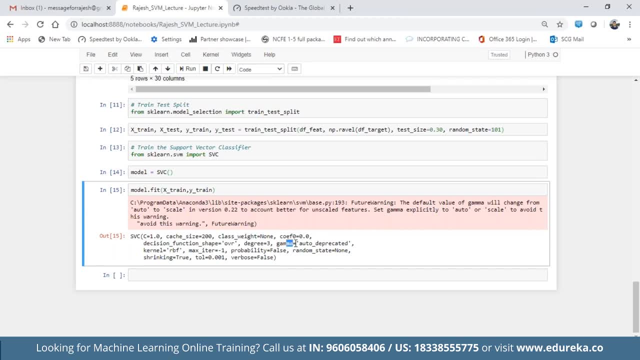 We will talk about two of them, which is C and gamma, but essentially it tells you what are the default values, the of the hyper parameters that it is currently using. and now, once we have trained it, now we have to start doing our prediction and evaluate how good the model is right. 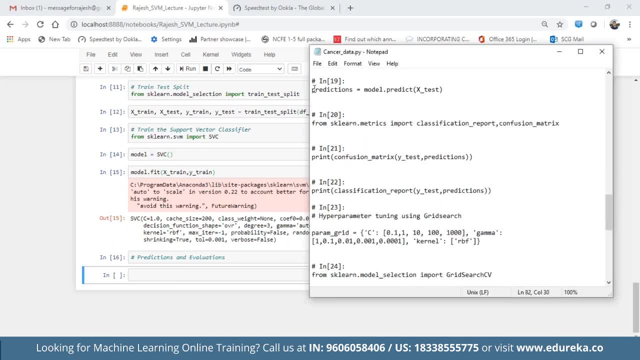 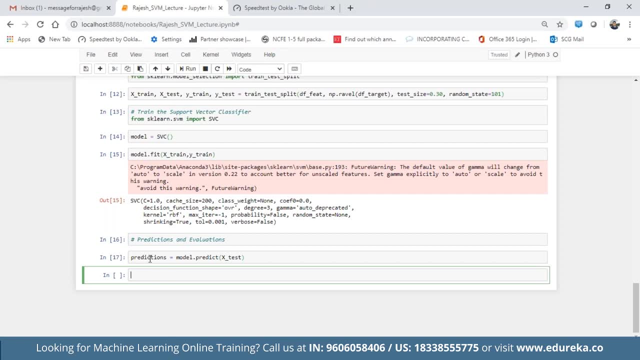 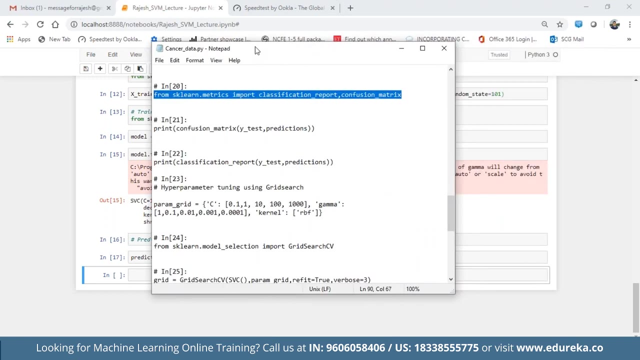 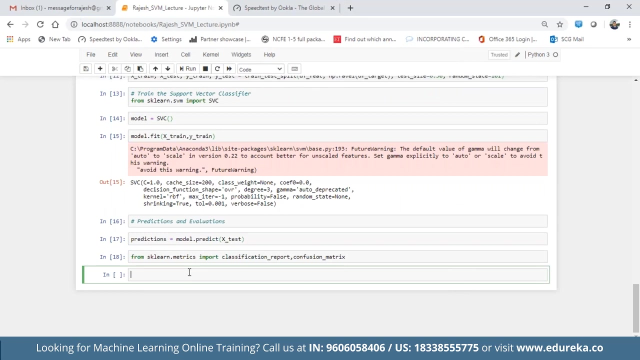 So what we will do is we will apply the model on the test data set- X test- and we have got our predictions in this variable call, And what we will do is, from psychic learn, We will import the metrics for understanding how good our prediction is using. 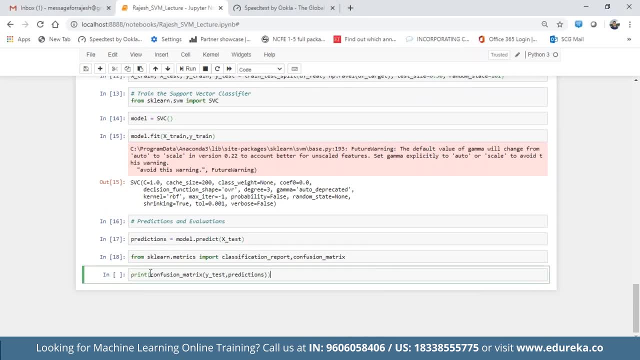 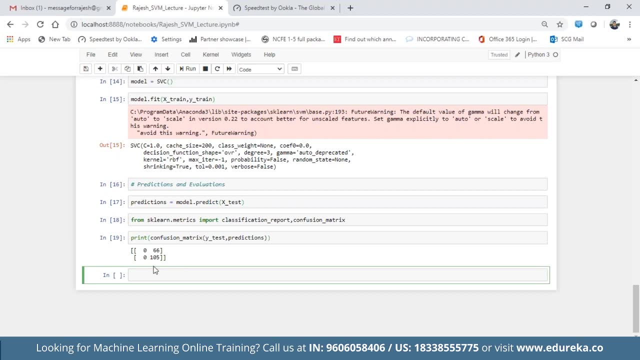 what we call as the confusion Matrix and the classification report. print the confusion Matrix. So here we see that actually the prediction is quite bad here, right? So all of the prediction is in only one class, which is that it is benign, and there is no prediction in the in the malignant class. 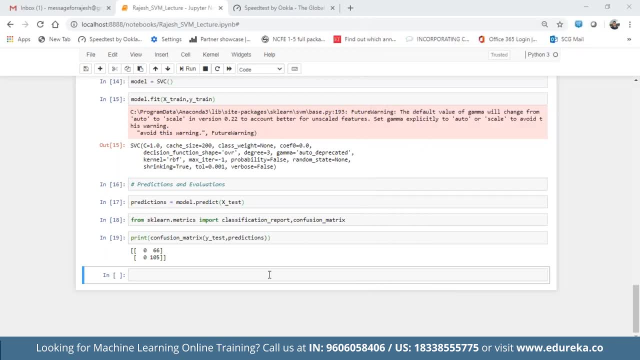 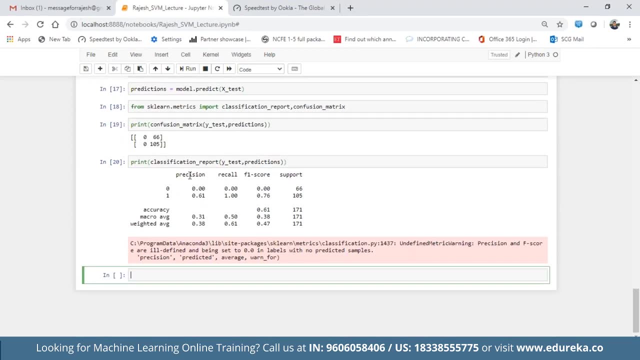 So that is the reason why we have to do hyper parameter tuning to be able to get improve the accuracy here. right, And if we look at the classification report, the precision, recall and F1 score, so precision is basically takes care of what is known as the false alarm or that you know. 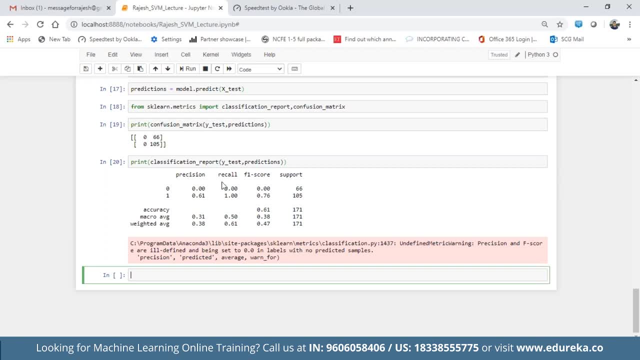 you have wrongly reported something as positive and recall Is basically: how much? how many of the true cancerous cases Did you act, were you actually able to predict? and F1 score is basically does a trade-off between precision and recall, because when one goes up, the other goes down typically. 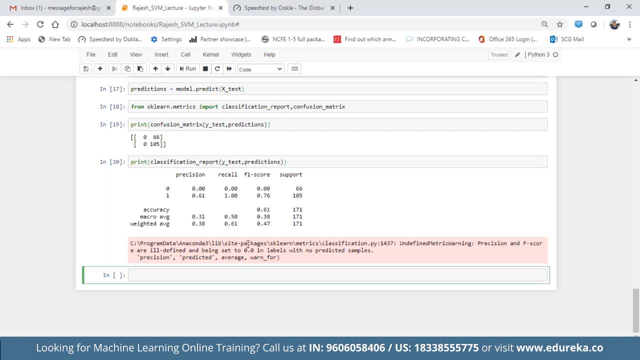 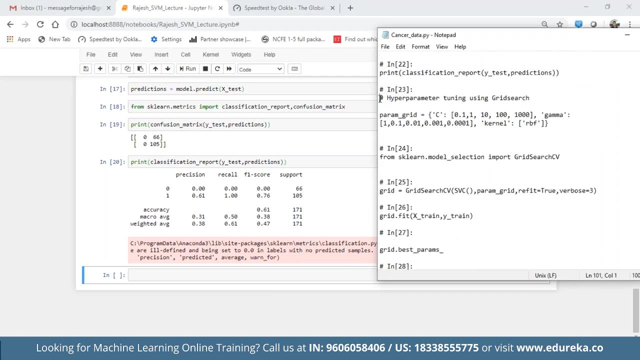 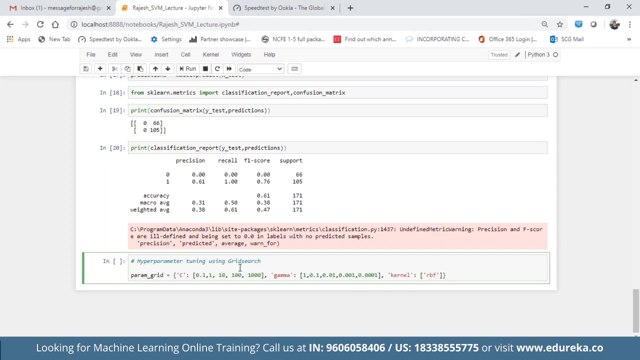 and F1 score is generally a geometric mean of the two. So we see that the accuracy is quite bad here and we need to do what we call as hyper parameter tuning. We will use a functionality within scikit-learn which is called grid search. 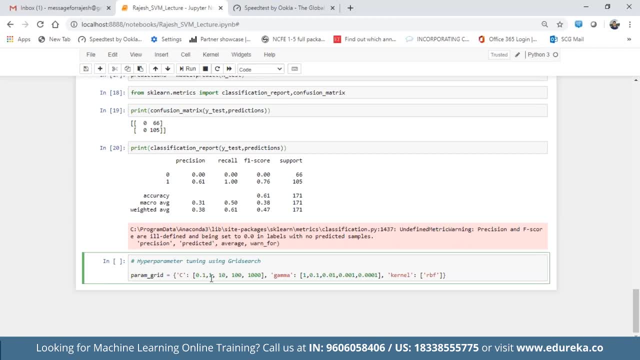 We will essentially look at two hyper parameters, which is C and gamma. another one. another hyper parameter is also kernel. So instead of radial basis function you can also use linear or polynomial right, But we are using RBF here and let's talk about these two right, which is C and gamma. 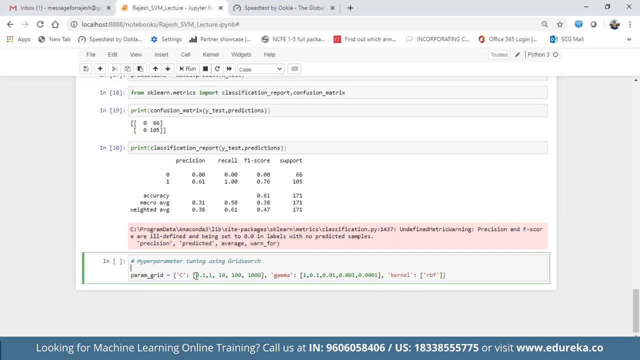 So C is essentially we are keeping from 0.1 to thousand here. varying it and see essentially is like a cost that you apply on how good your model is on the training set versus the test set. So if you want, if you keep the C value very high, 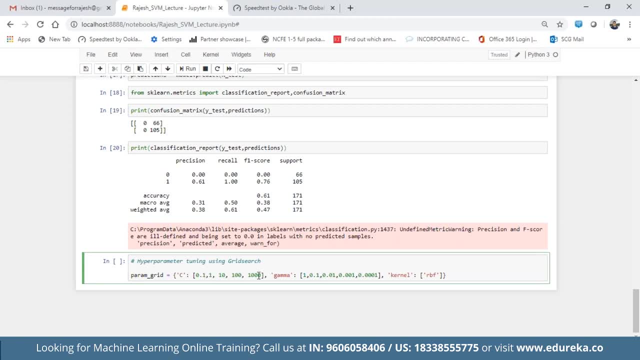 it means that you are more interested on your accuracy on the training set and not so much on the essentially. you you are trying to build a very complex algorithm which can divide the training data set Very well and the gamma is essentially the free parameter of the Gaussian of the radial basis function. 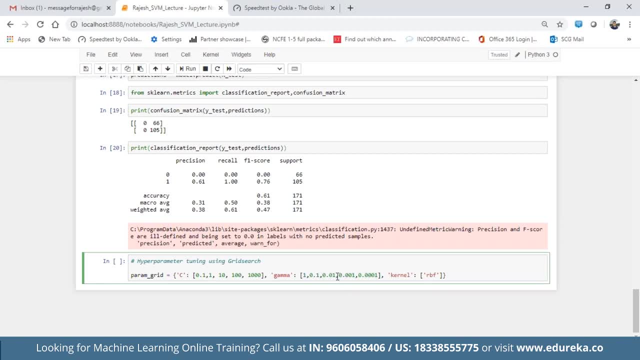 But essentially what it means is that if you increase gamma, the accuracy would decrease, but your solution time would reduce a lot. But if you decrease gamma, your accuracy will increase but the solution time also increases. So that is the trade-off: the gamma. So what should be the best value of C? 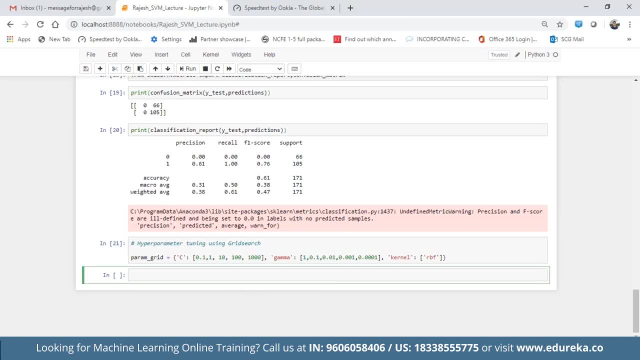 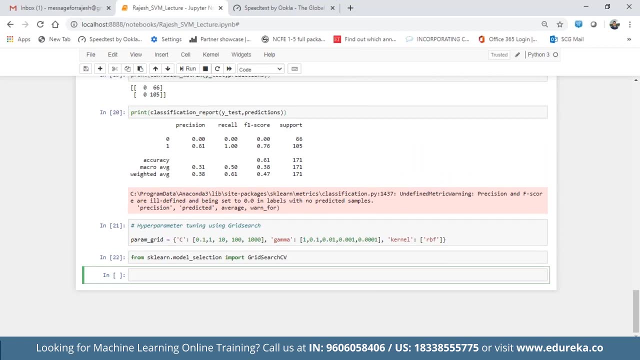 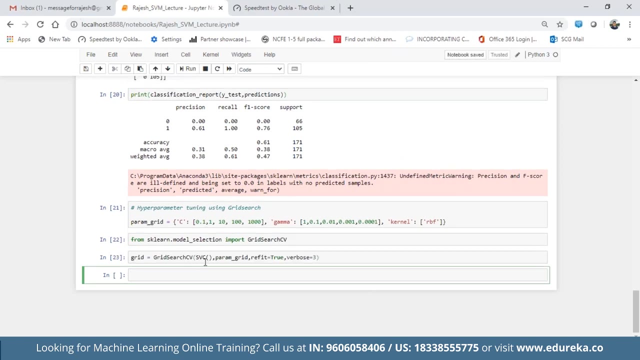 and what should be the best value of That is what we are trying to find out using hyper parameter tuning. We import the grid search CV functionality from scikit-learn here, And what we do is we assign to grade this particular grid search. 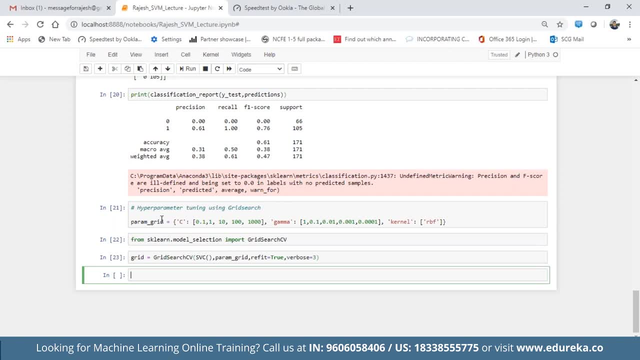 So we have called support vector classification model. We have given the hyper parameters values that we would like to be evaluated, and verbose is three just means that basically, it will show You some comments of what the scores are when it is looking at different values of these gamma. 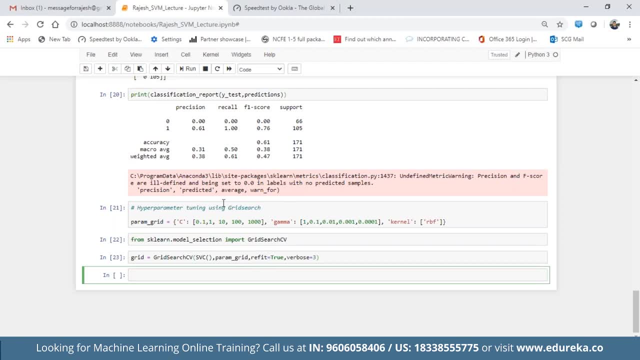 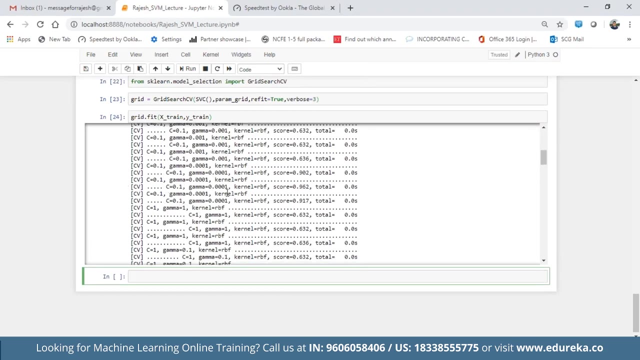 and C values and refit. true, just means that it will not only evaluate these parameters, but it will also refit the model, and with the best parameters. So now what we do is we run this fit on the training sample again And, as you can see, it is varying the values of C and gamma. 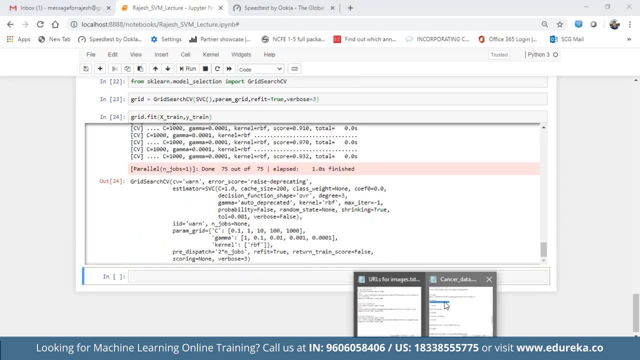 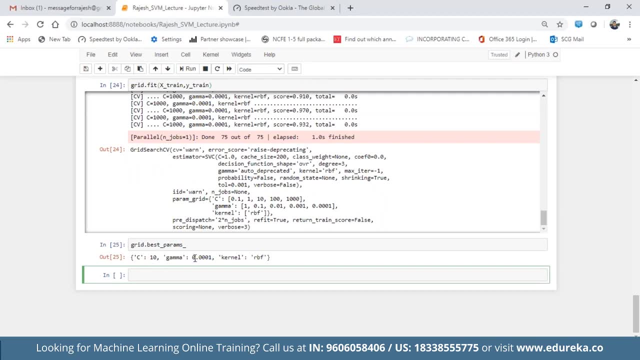 and finally it runs it. and now let's look at the results, right? So what is? what are the best parameter values? So the best parameter values are: C is 10, gamma is point zero, zero, zero one and kernel is RBF. That is what it has found. 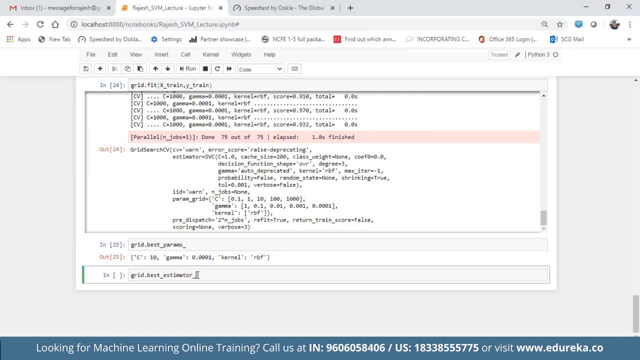 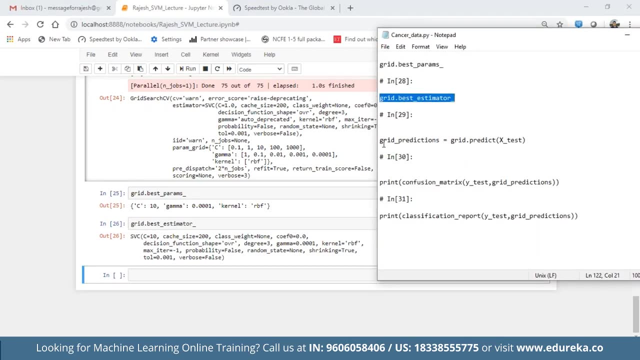 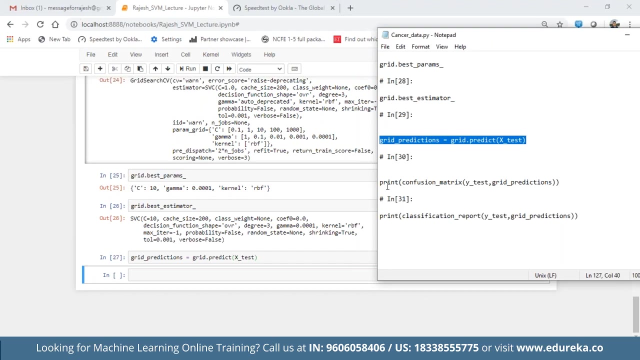 and then it can also give us the best estimator after having decided the best parameter. So this is the best estimator, as you can see, and now we will actually run on the test set using these, So test hyper parameter values and again check on the accuracy and the confusion Matrix. 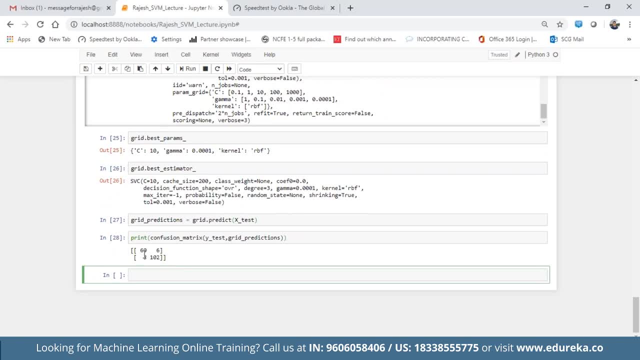 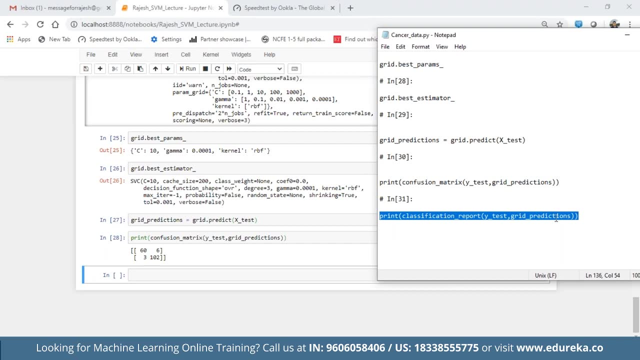 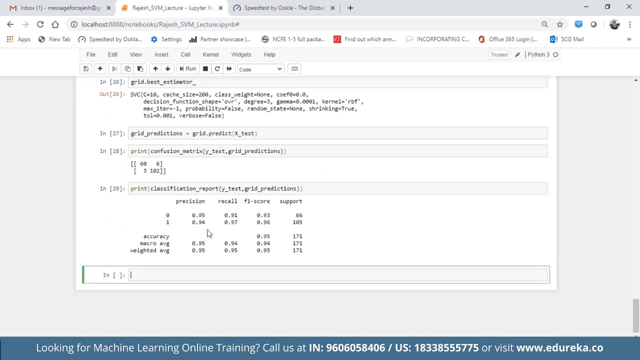 So, as you can see here, the accuracy improves a lot. right now You can see a lot of the predictions on the malignant category as well, and we will now predict the accuracy report as well. and you can see, now the precision has gone up to almost 94 95%. 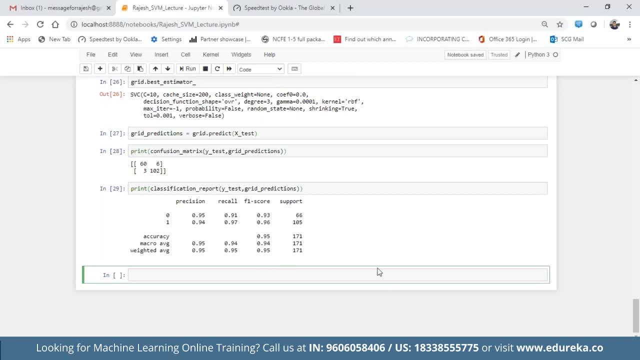 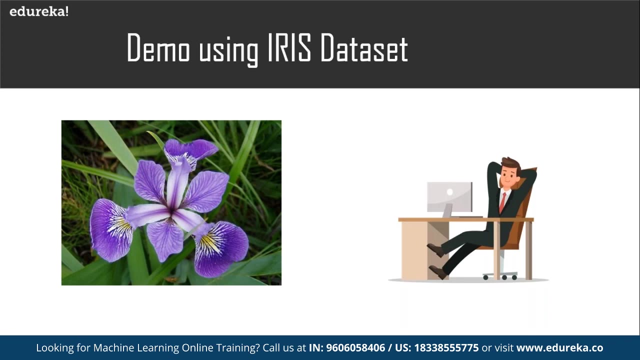 and recall is also quite high and have the F1 score. It's also quite high. So this is how we generally go through doing a support using support vector machine on on a particular data set, and I will also now actually take you through another example. 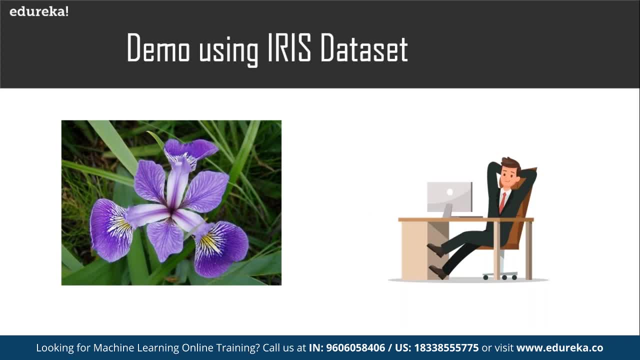 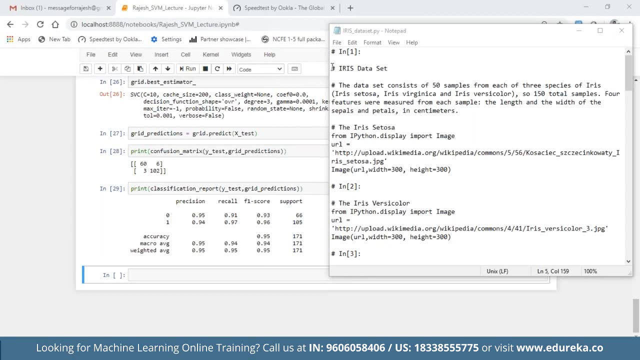 where we will use the iris data set. I think this is also something that you would have probably come across earlier in your machine learning work. This is quite a famous data set, which is a data set of iris flowers. So the iris data set essentially is, as I said. 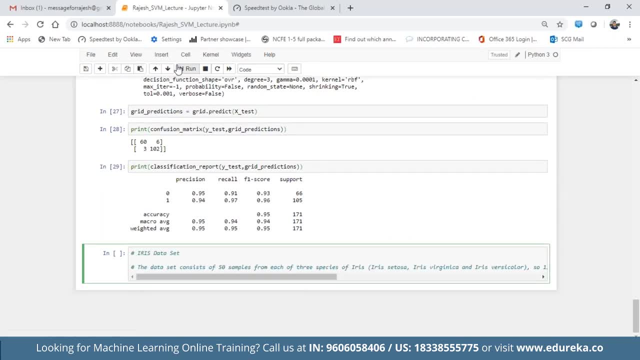 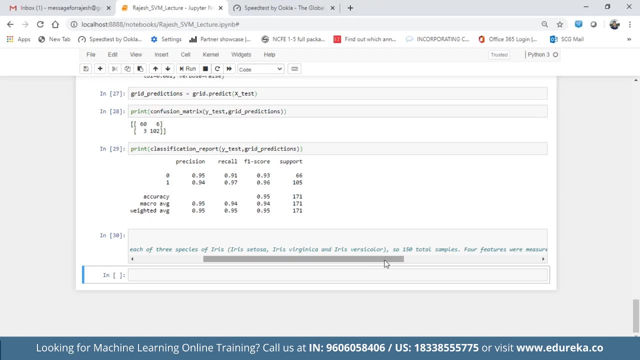 it is about the iris flower. There are three types of these iris flowers, which is basically the set: OSA, virginica and versicolor, and I will just show you how these flowers actually look like. So let us run the code here to basically. 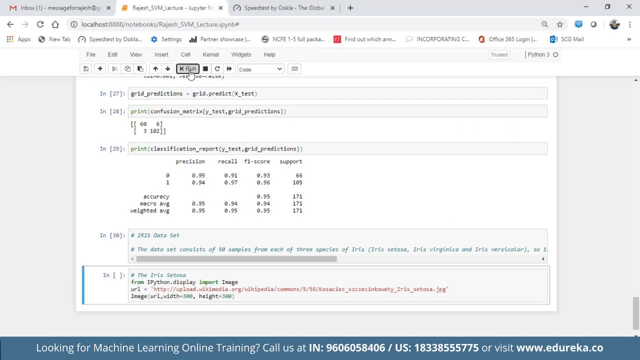 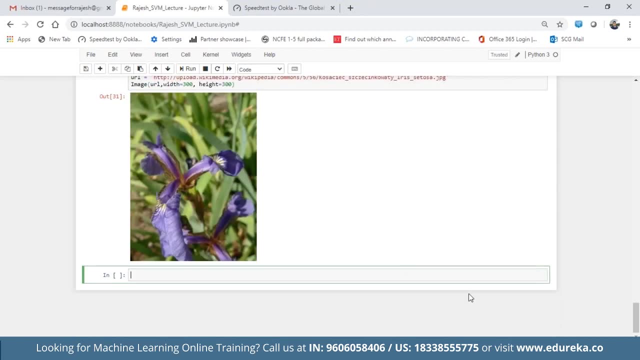 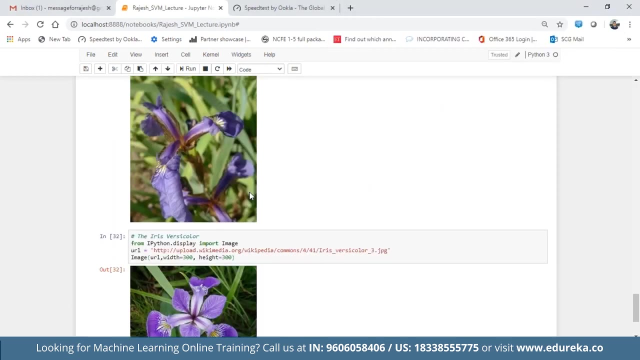 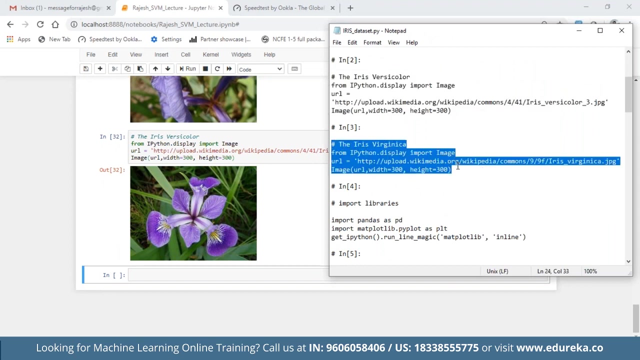 We plot those flowers from a internet source, So I'm just plotting or displaying this particular flower. This is iris set OSA, and now I'll just show you the versicolor as well. As you can see, this is versicolor, and I can show you the virginica as well. 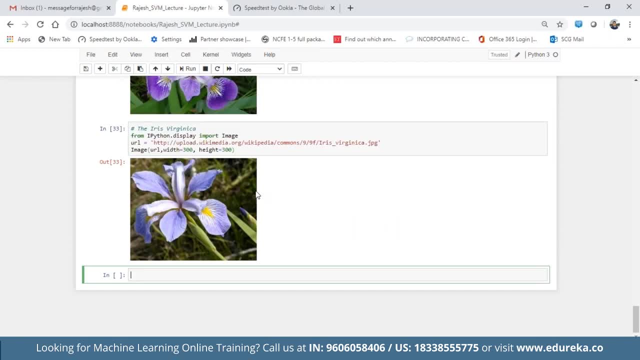 So we will go through exactly the same steps as with the cancer data. This is virginica. As you can see, all these three are of the iris flower types. There are these three kinds of flowers and we have data set which is 50 samples of each of these flowers. 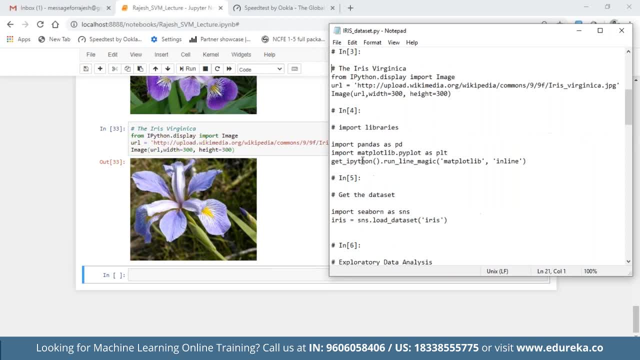 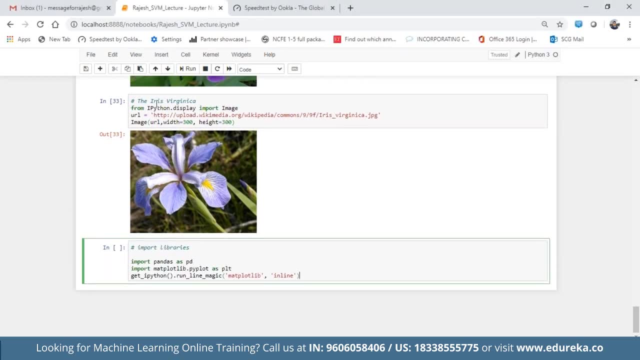 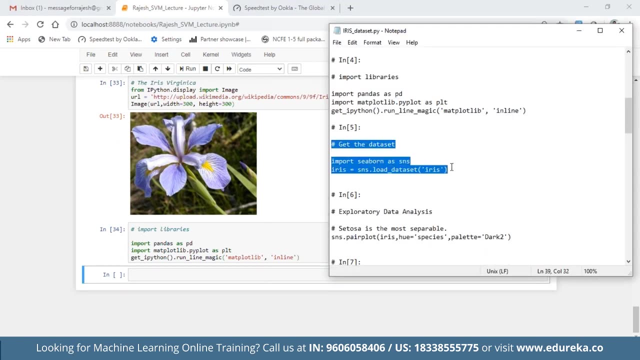 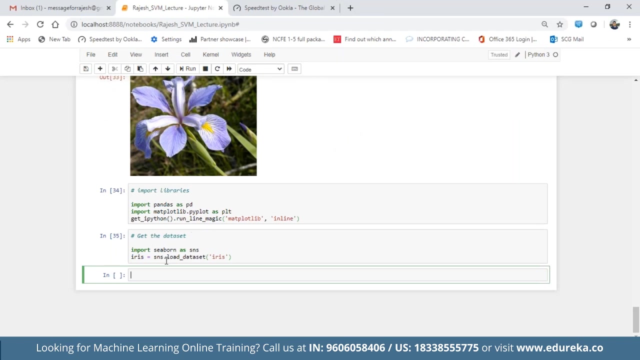 So there are 150 samples, and what we will do now is basically run through the same steps. So we will import all the libraries as before And get the data set, and in this case the data set is in a package called seaborn. seaborn is a visualization package. 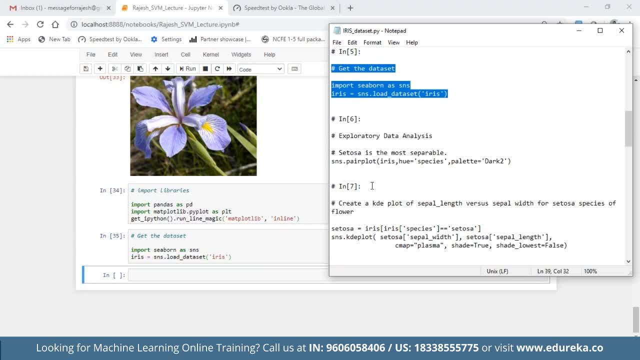 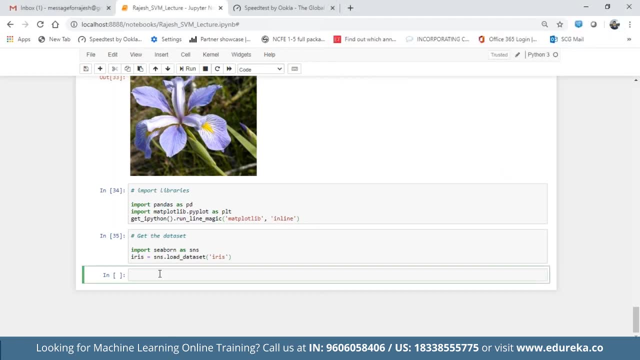 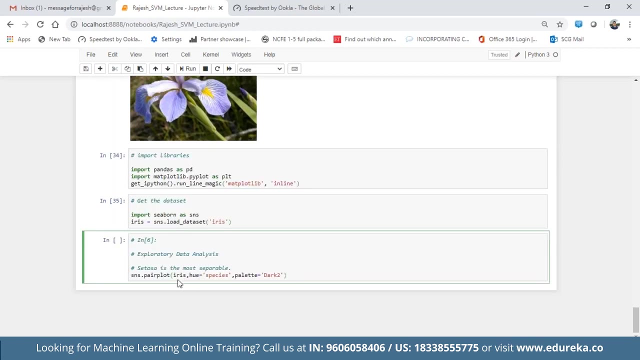 which we will also use to do some exploratory data analysis. Typically, you can also do exploratory data analysis using other packages like matplotlib, even within a python itself. There are other ways to do it and many other packages are there. So we are trying to do now. 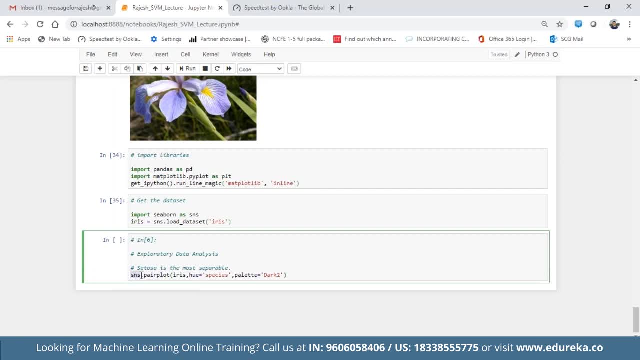 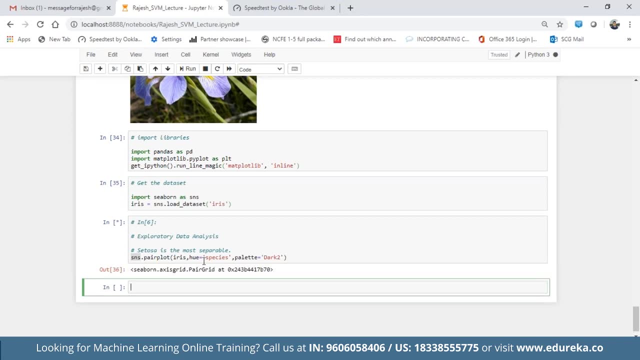 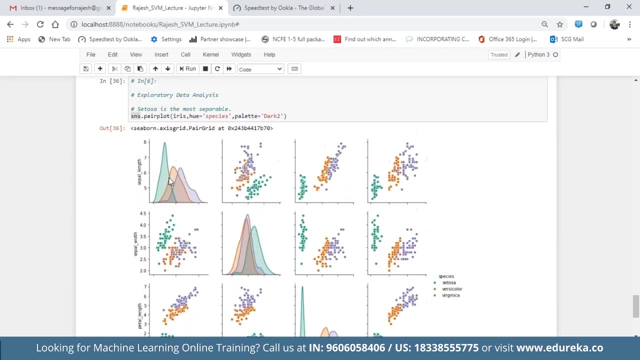 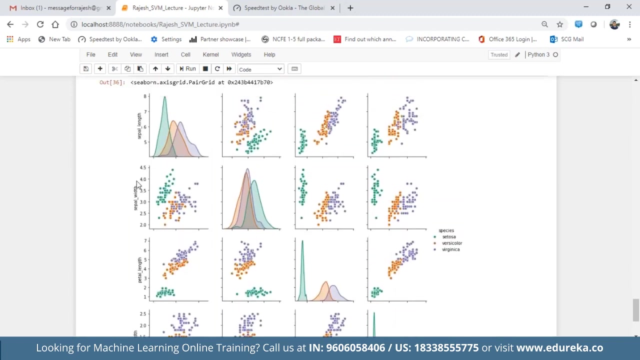 A pair plot using the C plot package and let's just run this and we will be able to see the. yeah, So, as you can see, this is a pair plot, So there are essentially two features of a flower. So it is the, basically your petal, and your sepal petal is your, the colored part. 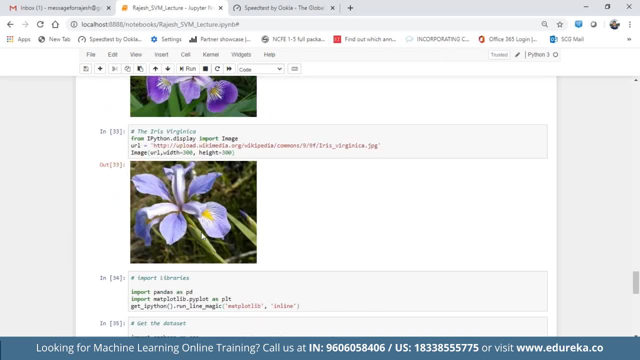 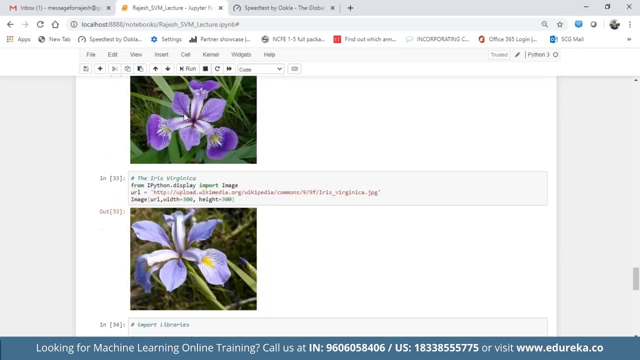 and the sepal is a green part just below the flower, right, which is basically: this is the sepal and this is the petal part right. So what is the length and width of the petal And what is the length, length and width of the sepal is what 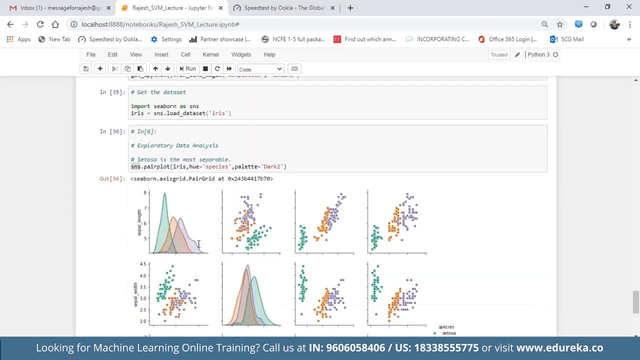 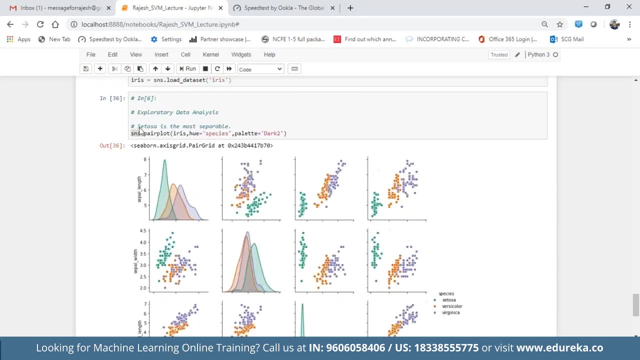 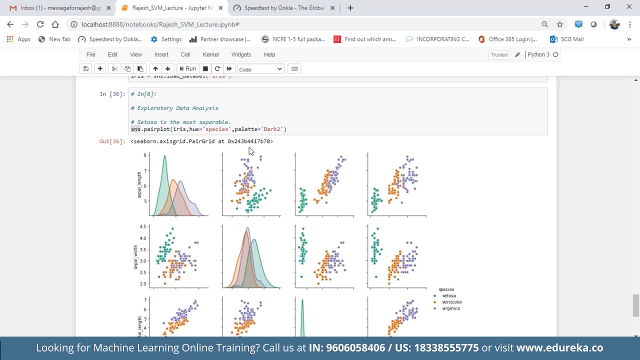 can help us to classify these three kinds of flowers, And that is what we are attempting to do using support vector machine. So, as you can see, this, this pair plot is telling us if we plot sepal length with respect to sepal width, then what kind of plot? 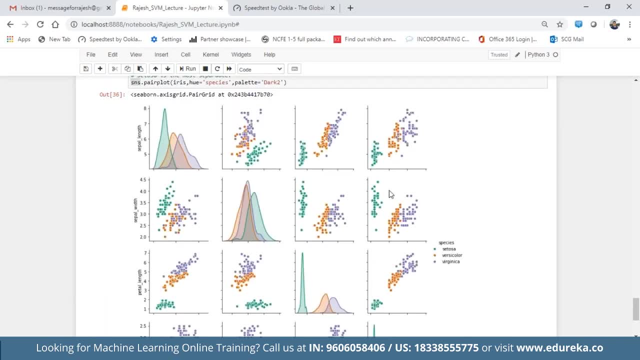 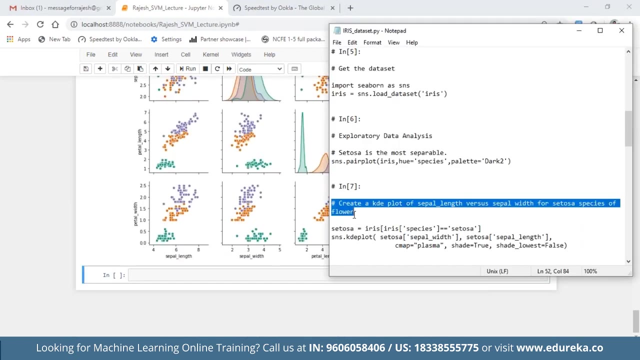 We get and you, as you can see, this green color is basically your setosa. So we can see that the setosa is quite different from the other two, which is versicolor and virginica, and it is quite easy to classify setosa. So let us create a kernel density estimation plot for setosa. 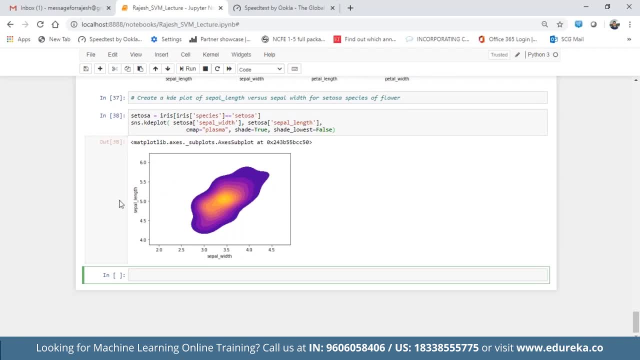 And let's look at that. It is of the type which is quite easily separable, right? So we can see that if we plot the sepal length and sepal width of setosa, we see that this is the kind of plot we got. 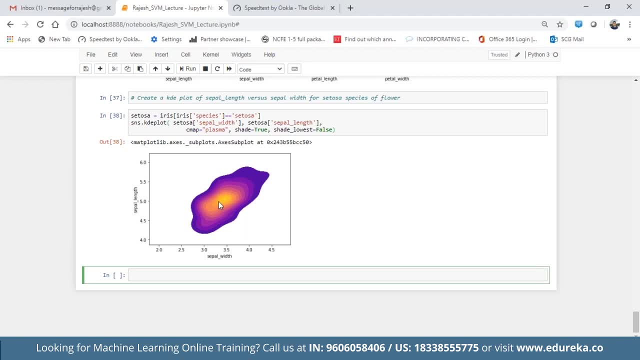 So the density of the kernel is maximum at the center here and then it decreases. So we see that it some kind of a linear relationship is there between these two, And now we will actually do the same steps to classify these three. So we are going to run. 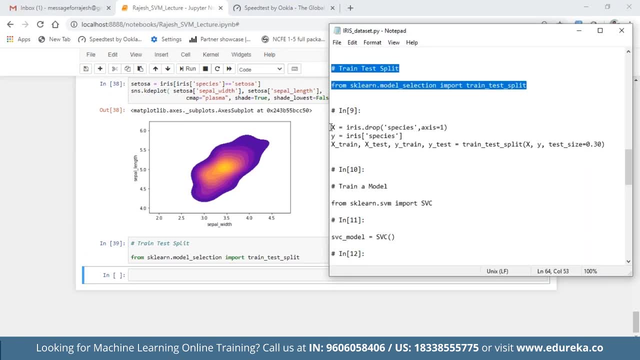 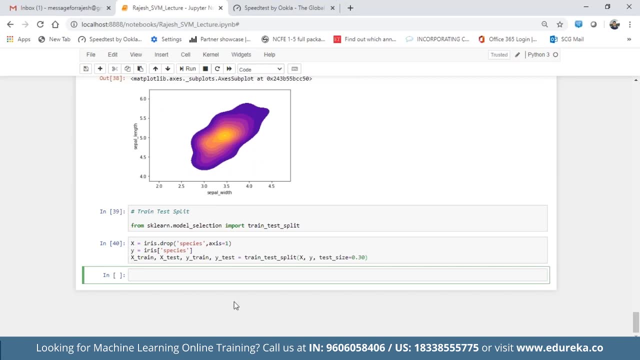 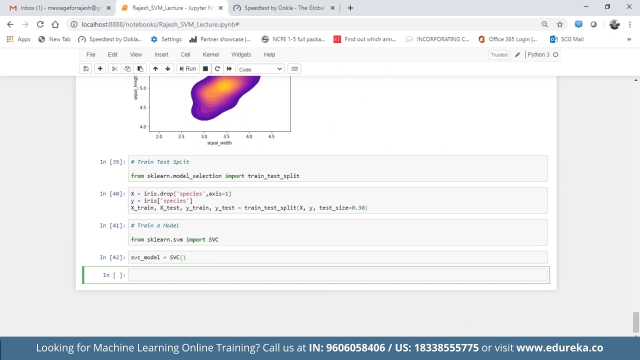 the train test split from scikit-learn and we are going to assign 30% of the data set to test and the remaining to train. Here now we will import the support vector classifier and to train the model, Initializing the support vector classification model here. 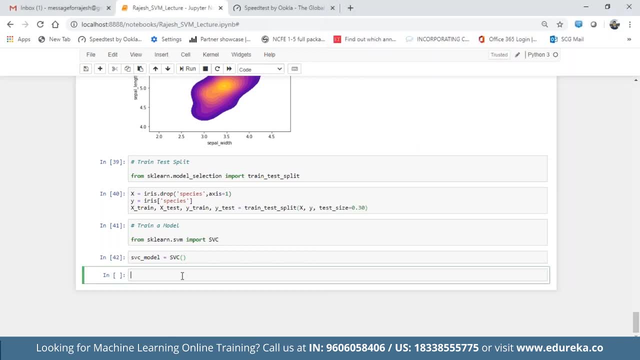 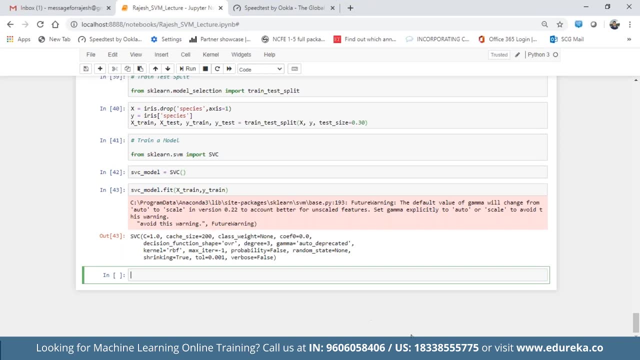 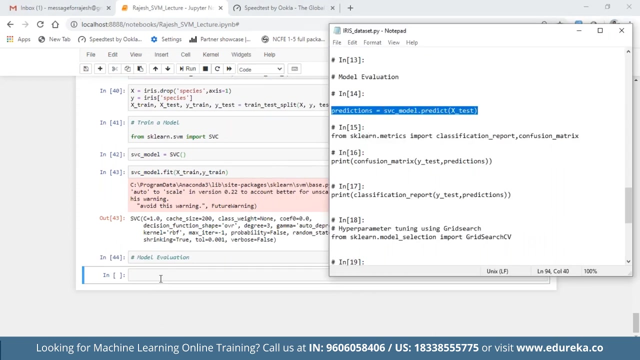 We are now fitting the model, So all the steps are the same as we saw earlier in the cancer case. So this is with the default setting. Now we will do the model evaluation. So we are now building the predictions after having run the training model. 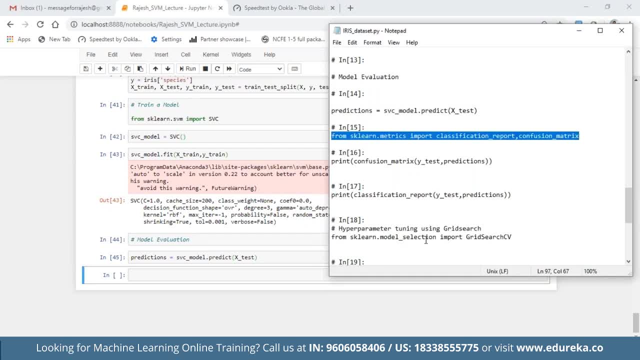 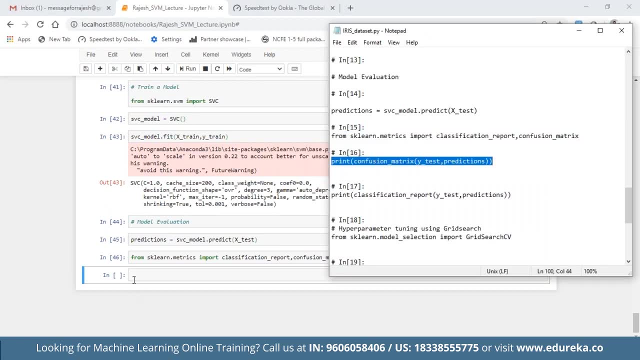 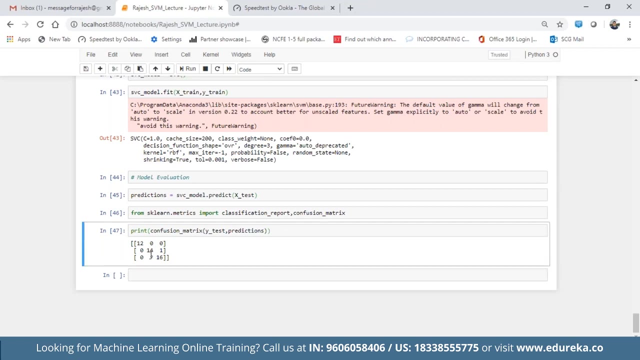 on the test. We are running the prediction and now we will plot the metrics for accuracy. So if we plot the confusion Matrix, we see that it is the accuracy is already quite good. So we see some misclassified samples here and here. And if we run the accuracy, 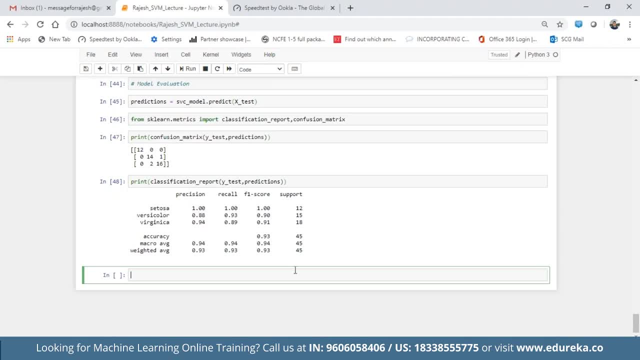 we get the classification here. So the obviously that the precision, recall and F1 score are all are quite good. Now we can do hyper parameter tuning, but it will obviously not improve the result too much, but it can. let's see if it can improve even a little bit. 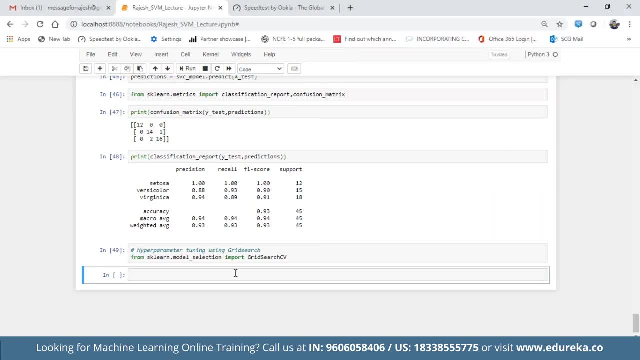 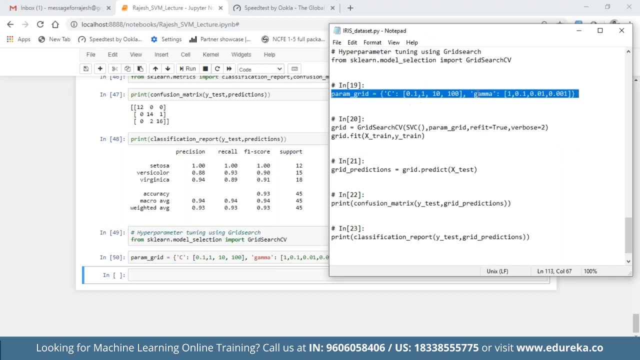 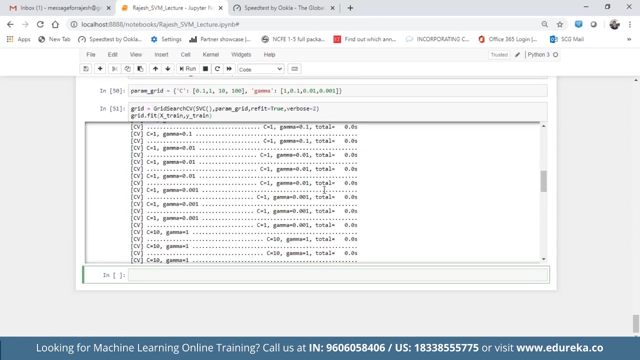 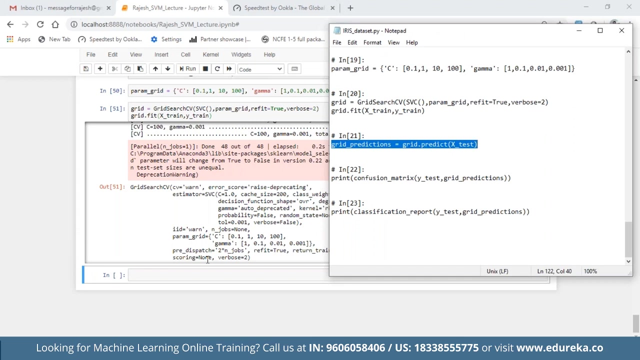 or not right. So we again run the grid search for hyper parameter tuning. the C and the gamma values are between these values that we saw and we run that and it shows that how it is checking for the best hyper parameter values. And now we run the grid predictions. 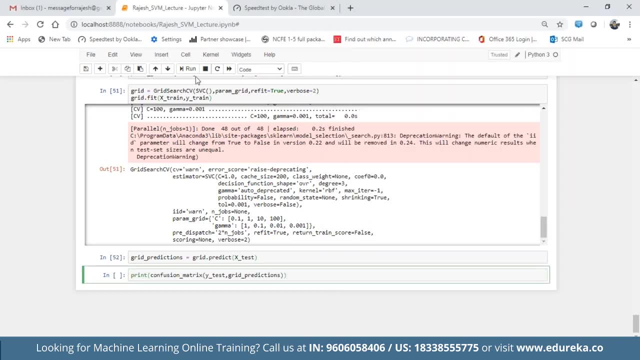 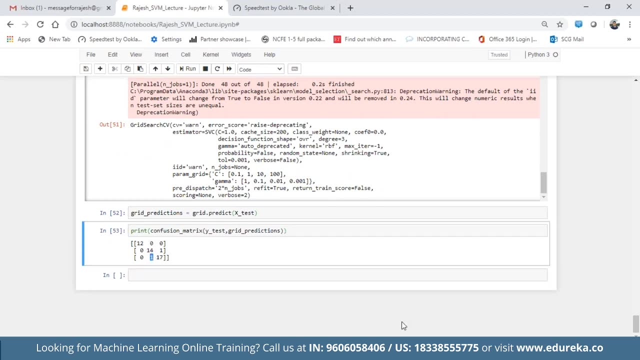 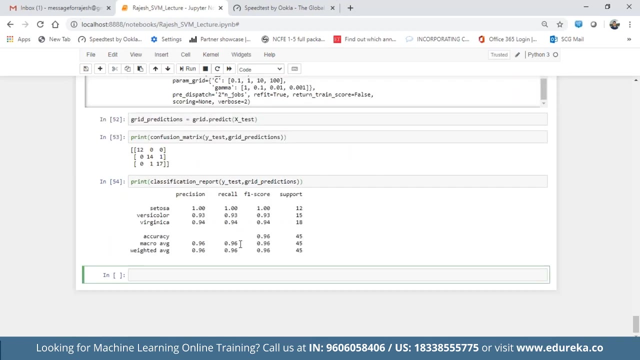 And after doing the parameter parameter tuning, let's look at how the results are. So we see that almost the result is the same from here. Actually, one more sample got classified correctly, but all of the others is kind of same. right earlier Also, the result was already pretty good. 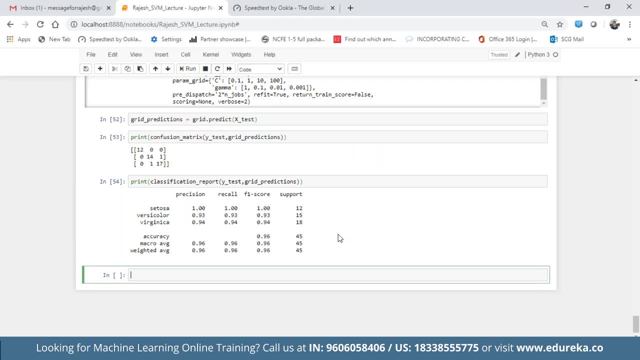 So it improves the result a little bit, but not so much So. in some cases hyper parameter tuning might be very essential. in some cases It may not be that essential. Now let's look at what are the advantages and disadvantages of SVM right. 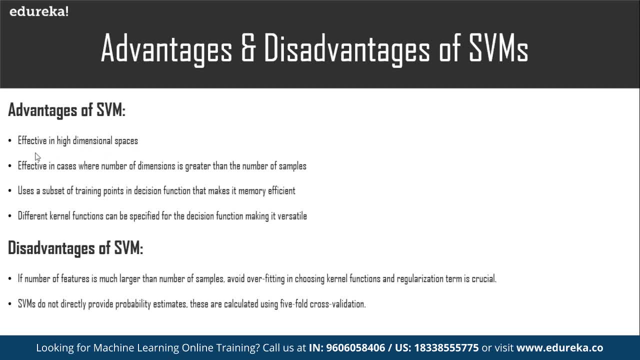 So we saw that SVM is quite useful and effective in high dimensional spaces and specially in cases where sometimes the number of dimensions may be greater than the number of samples. This is quite useful and we only use a subset of the training points for the decision function. 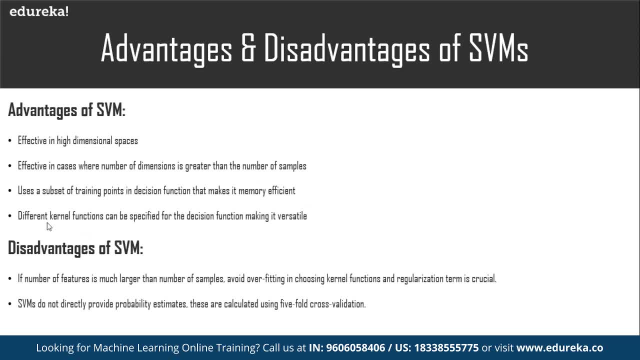 Therefore it is quite memory efficient and different kernel functions can be used, like, for example, linear, radial basis and, and, and polynomial as well, and. but so there are some disadvantages. disadvantages is one is that there can there are chances of overfitting if we don't choose the kernel function. 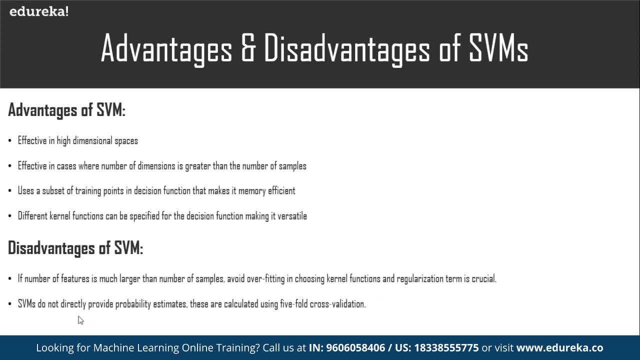 and regularization term well, so, which is quite crucial, they- so SVMs- do not give us probability estimates directly. So some of the other techniques, like decision trees, etc. They will give you a probability Estimate as well, which is not there in case of SVMs. 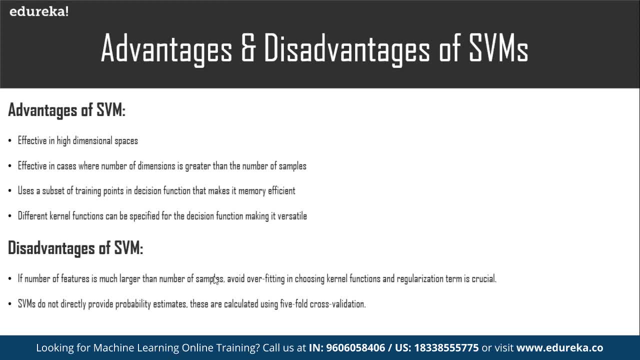 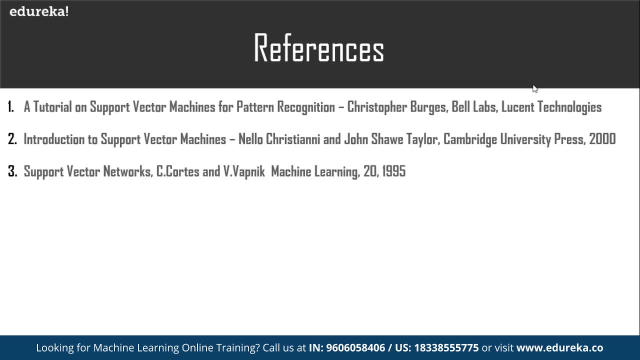 And if you have to get probability estimates of each of the classes, then we have to use the five-fold cross validation. So these are some of the references that you can look to. the first one here is a tutorial on support vector machine for pattern recognition by Christopher Burgess from Bell Labs. 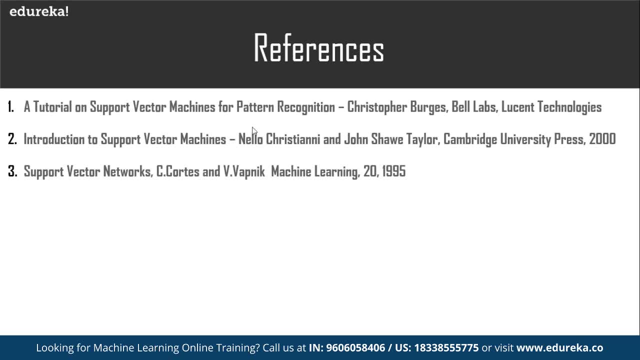 This is something that I found very useful. There is a book called introduction to support vector machines by Christiani and Taylor by Cambridge University Press. This is also a pretty good book on support vector machines and the original sort of. one of the creators of support vector is vapnik and he has a paper. 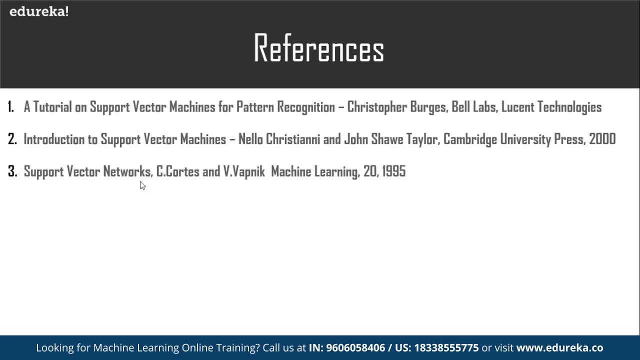 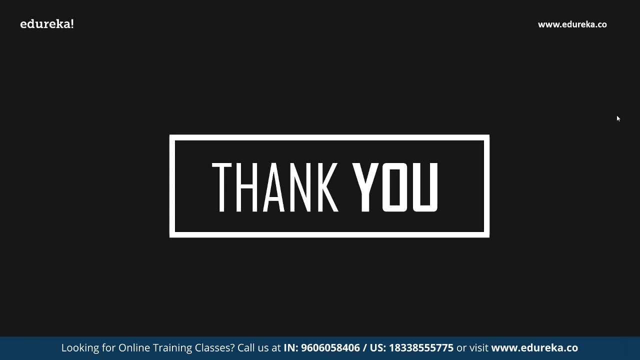 in a journal called machine learning, called support vector networks, And this is also a pretty good reference. Okay, so we come to the end of this particular session. Thank you, Thank you very much. Thank you, Thank you.